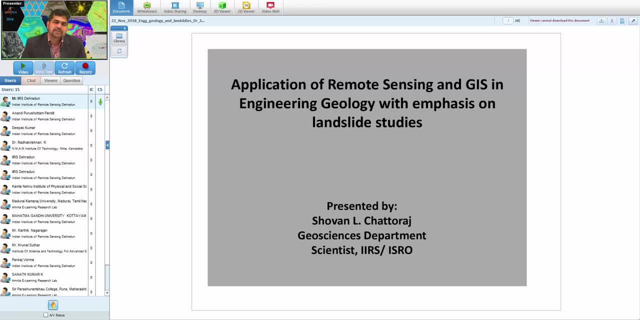 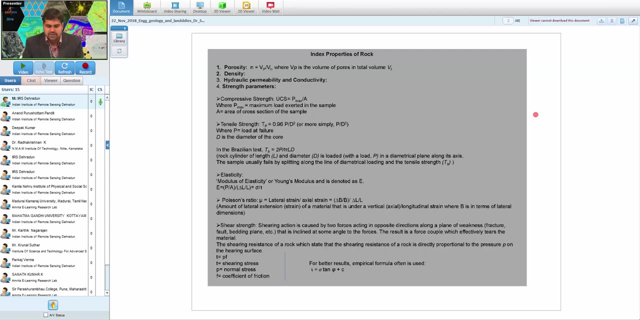 sensing and GIS technologies and we'll try to see how we can solve engineering, geological problems and, more importantly, the landslide studies. So to start with, let us understand first few index properties of rock. few of the properties. that is important. This is important because 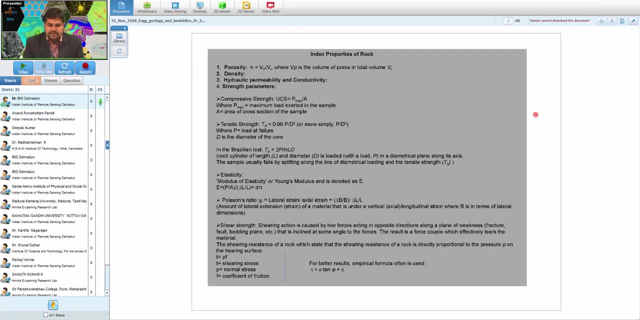 without this we cannot proceed further, and this is the mainstay of any engineering geological work. So what are the index properties of the rocks, If I keep the porosity, density, hydraulic conductivity etc. apart? I hope people already understand that. Let us come on to the 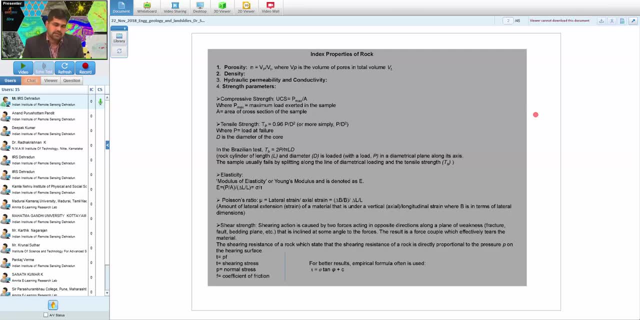 strength parameters. So there are three things that we need to understand. One is stress, another is strain and the third is strength. So these three parameters, clearly, if we understand, we will be able to grasp other things also. So the strength is suppose it's basically stress is basically your force per area. It's basically, it's the same unit as pressure. Pressure is also force per area, but then what the difference is Different lies in the fact that your pressure is force per area and stress is force per area, where limit a tends to zero. So 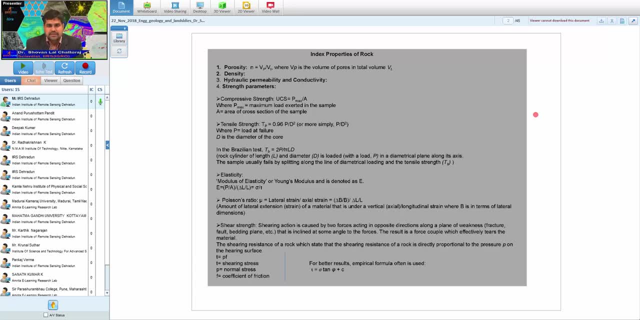 area has to be close to zero. So that's what it is. If I apply force on an infinitesimally small point, so that basically will indicate it'll give me the stress projected applied on that point. So there are three types of main stresses: stress regime that we're going to discuss here, or the engineering. 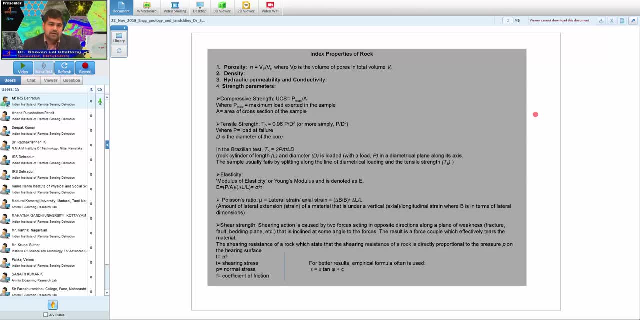 geology as such is concerned with. One is your compressive strength. So that is normally if I press a surface, put a vertical pressure on that vertical force on that, so that becomes my compression And secondary stress. And second is the tensile stress. Tensile is if I pull that apart. So first is pushing like this, Second is pulling that apart will lead to development of a crack once the strength of the rock is superseded. So that basically is tensile stress. 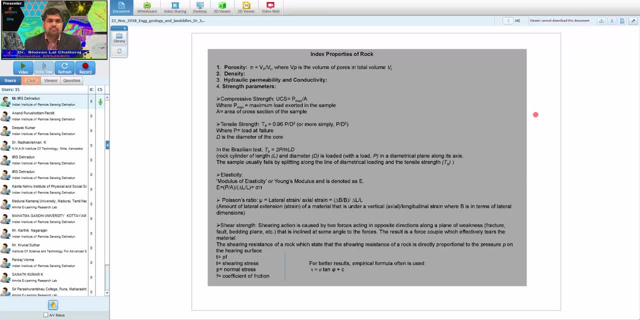 Next comes the shear stress. Shear stress is mainly concerned with your landslide studies because the shear has to fill between the surfaces for a landslide to happen. So among these three, shear stress is of utmost importance for landslide studies. Accordingly, connected with these three types of stresses, we have three strains. So strains are basically development of distortion. So the distortion may destroy the surface. So the entwined stress may not destroy the surface. So the heavy tail kind of dry stress can destroy the surface of the sand. So the transform is lower and the çevre stress can destroy the surface. So we mind is not as affected by this, since it is relatively less stressable, which will lead to decrease of pads. So GI gospel advise. 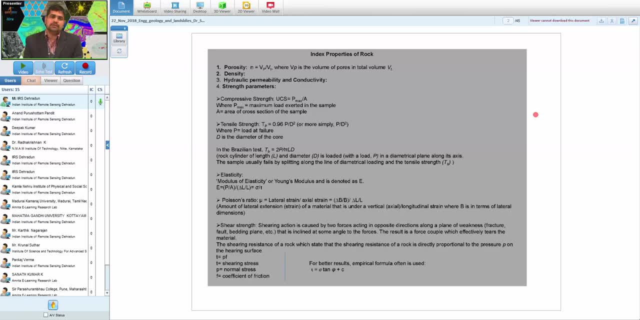 be in the form of a linear feature. so we all know that class 10 physics example why there are gaps between railway tracks so there will be expansion because of the heat in the summer and so gap is to be returned so that it can be accommodated. the increased linear length. 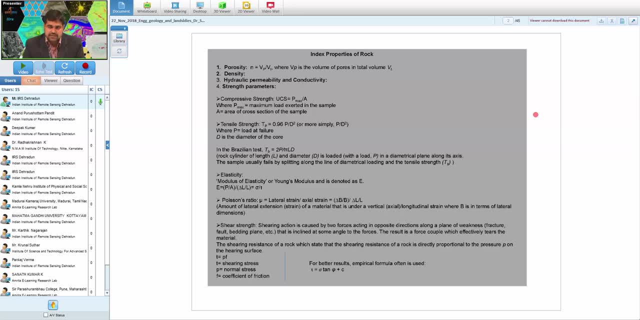 is accommodated. so increase in linear length is strain 1, then strain 2 can be. suppose change in the volume, the cube as such can be reduced to volume. increase in volume if I change the density right. the third can be change of an originally right angle. so if I into D, suppose we think of 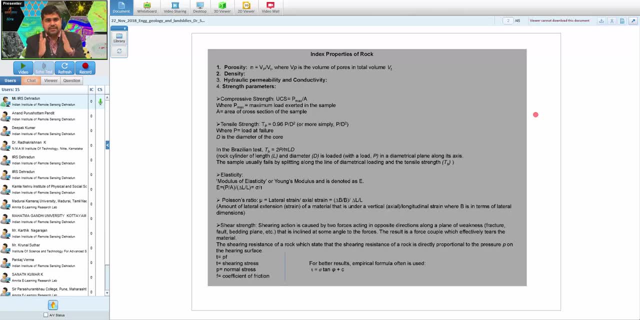 a rectangle or a square and if I change this into a ROM, so that basically is change of originally right angle. so these three type of strengths are there. the strengths are the deformities and once you, the strain progresses up to a certain distance that it cannot regain back to its original shape. 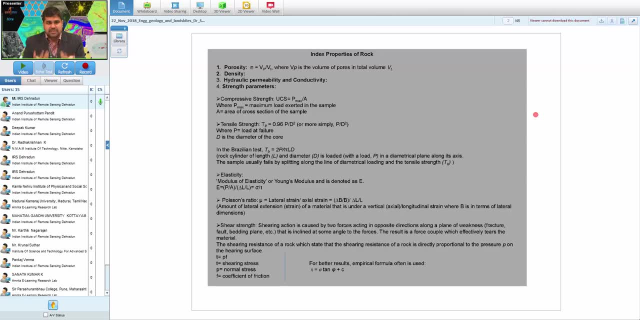 so we mean that the strength has been superseded, strength of the material has been superseded. so here mostly we'll discuss about the stresses. now, as I have told, the shear stress is the stress that is the most important. we have discussed about the compressive strength, the tensile strength. 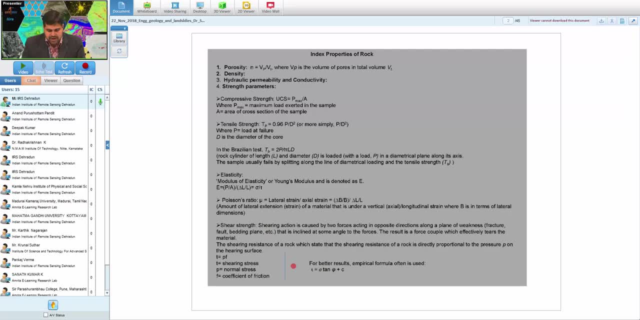 and the shear strength. shear strength is the stress that is the most important. we have discussed about stress. now we have discussed a littletur. eh, here we had described the shear stress, my respect for the JImeter stress, so yi is the right column, five by one here in summary for sm at seven. 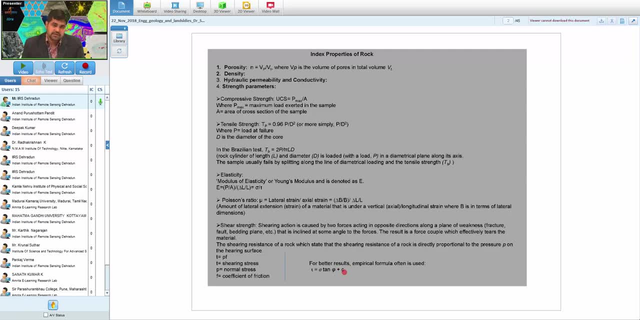 x, z, yi is the stress of shear stress. this is about tired, ready strength and today's term in terms of the shear stress here in general, the shear stress. the stress is called the cost of shear stress. if we take the shear stress, we can say: now that you touched upon thew should. 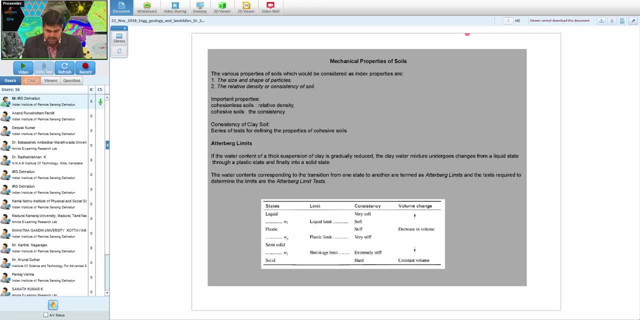 continue with this. let us come to the first slide. the second slide- rather earlier slide we were discussing about the properties of stress, strength and strain, is mostly related with the rocks. now come to the soil. so soil also have different types of properties, engineering properties that are required to be studied. so let us first talk about the size and shape of the particles and 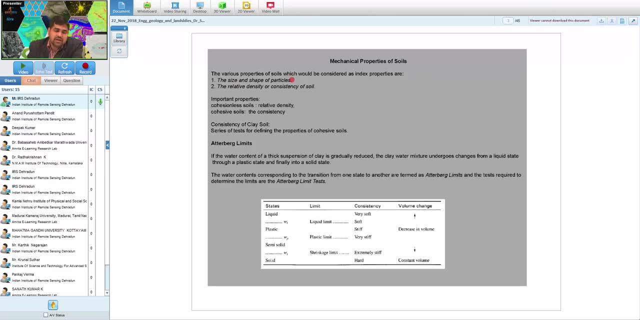 then the relative density and the consistency of the material. so consistency of the soil is really important, is a really important factor in terms of as far as the strength is concerned. so cohesive soil and cohesion less soil generally these two soils type we get, obviously if you go. 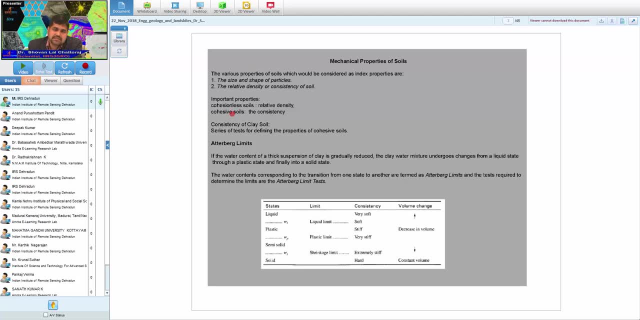 to the beach and take a beach sand. there is no cohesion as such. that will be cohesion less soil and a clay soil and mostly clay particle, so there is adhesion between them so that clings to a surface. so that is a cohesion less soil. so that is a cohesion less soil. so that is a cohesion less. 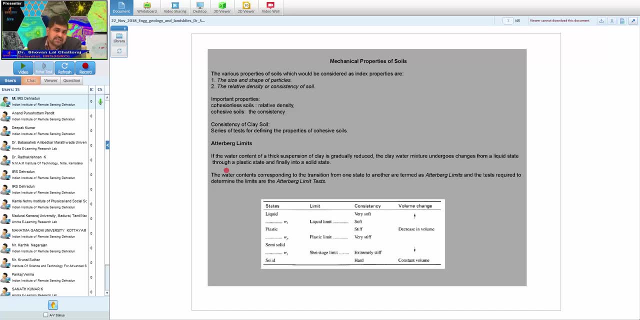 soil. so that is cohesion. well now how to describe the consistency of the two types of soil. cohesive soils is what we can change. we can check it's consistency by Atterberg limit. attractive 했는데 is a scientist to define different limits for testing the consistency of cohesion soils. so 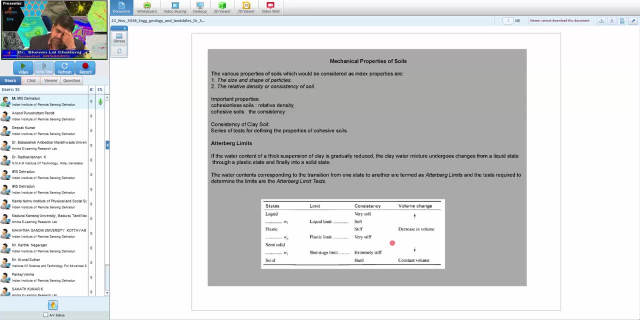 let us take a clear lump, as we started with theслиinklingmanship load of moisture. so that is almost close to a liquid state, and from the liquid state, if the water is extracted out continuously, it will, once upon a time it will, reach a solid state. 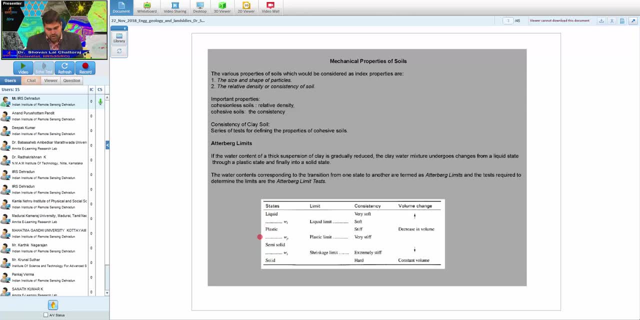 Now in between we have these two most states developed. So one by one I will come to that. So if the state of the clay lump, suppose, is close to liquid, almost liquid, so consistency is very soft, then if I heat that up, so evaporation happens of the water content, so the material. 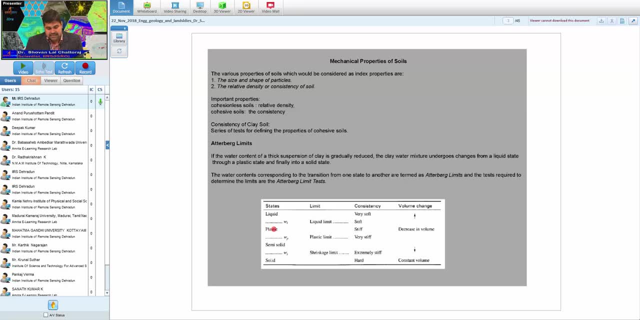 becomes slightly stiffer and the state will be plastic Again. heat it so that will be close to semi-solid state. It will be very stiff and once it reaches the solid state it will be a very hard substance. Please understand if I extract water continuously. 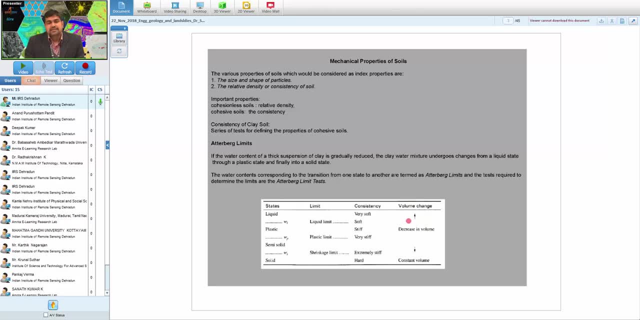 from this liquid, This liquid state. so the decrease in volume has to happen because water is going out. So ultimately, when it reaches the solid state, there will be no change as such after that, because it has all my moisture has gone out Before that. there will be continuous decrease in volume from this point to that point. 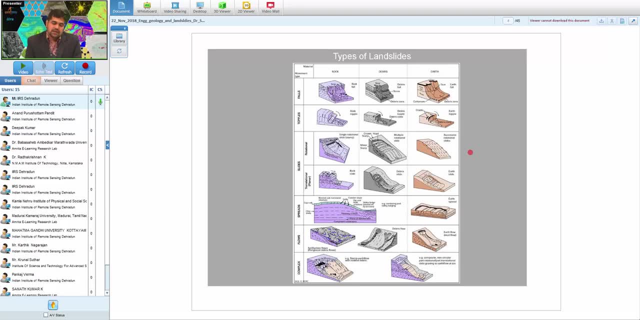 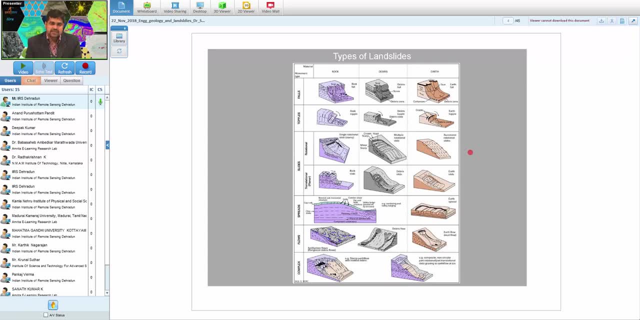 We are, landslides are a big umbrella term. We are, landslides are a big umbrella term. I will explain what kind of landslide is and the 배�� you mentioned there, Because on exams of outcomes you shouldn't do that. Because on exams of outcomes you should not do that, Because on exams of outcomes you shouldn't do that, Because on exams of outcome you shouldn't do that. So land slides are essentially called versions of landslides. So land slides are essentially called versions of landslides. So land slides are 진짜 consisted ofulates, so treatments oflings, So we call them land slides as such. So we have to pay attention, we have to understand the different classes, different types of landslides. So first in this, in this axis, if you see I had taken the material involved- 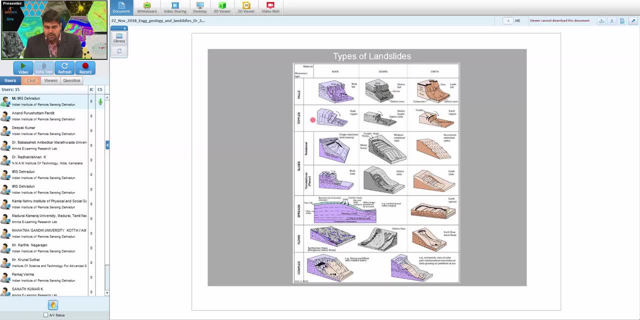 so material involved. rock, it is big debris, or it is earth. Earth means nothing but soil. rock fall or a earth debris fall, then topples. so what is the difference between fall and topple? fall is just a fall. rock is falling from a you know uphill and then topple is along a discontinuity. 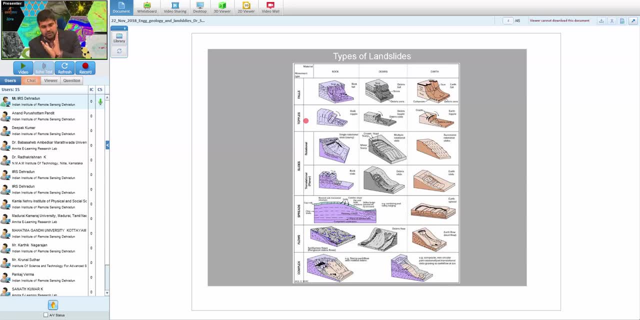 plane, the whole whole thing is toppling down. so along a discontinuity plane- the detected plane is the already defined discontinuity- may be a joint in rocks, so similarly topples happen in rock debris and earth topples. next comes the sensu stricto: slides as such. so slides can be of 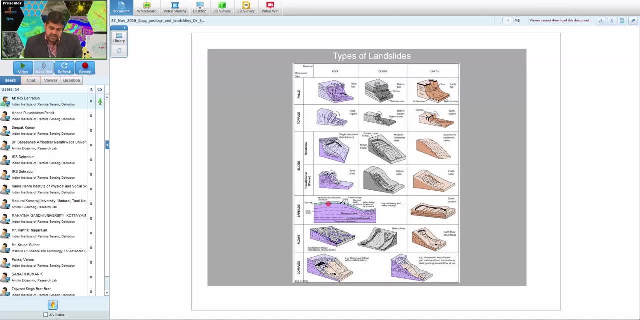 two type: one is rotational, another is translational. so in rotational slide the failure plane will be this, like this curved one, and translational soil it will be a planar, one straight plane. now there are other types of slides, like spread. spreads are nothing like you know. the whole thing has spread. 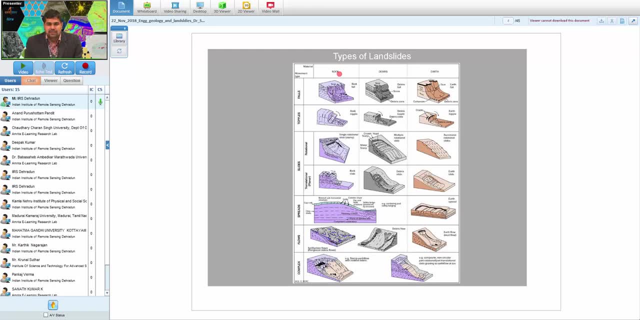 so it can be. rock basically cannot, you know, spread, but debris and earth can. next is flows: flows. typically we get earth flow or debris flow, very common rock flow as such is difficult to happen, physics wise, or engineering geology wise. now, in any big landslide there will be always a complex. the last class tells about the complexity. 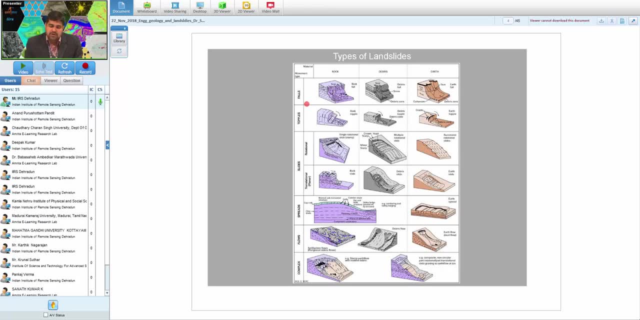 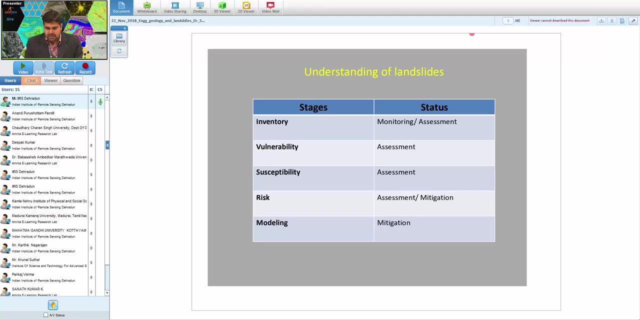 of the phenomenon. any big landslide, if you think it will not be purely fall, or a purely topple, or 46 together- is to be defined, is to be separated clearly so that we can identify each part clearly. so how do i understand waterbot? understanding of landslide is not a 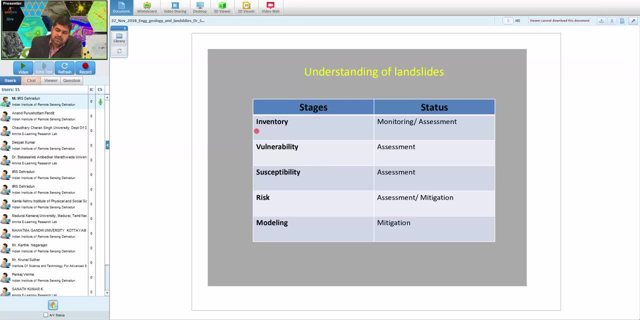 landslides with landslide studies involves using satellite remote sensing technology. technology suppose it starts with making the inventory. so what an inventory is? basically, it is the landslide polygons that you can detect by visual estimation or by digitally on a satellite image. so the polygons you have to make the safe files, so that becomes my inventory. then I come to the 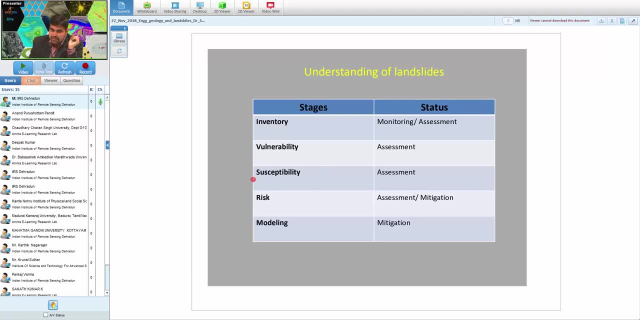 vulnerability calculation, then comes the sustainability map preparation and then the risk. so risk is obviously a tick excuse of vulnerability, susceptibility and other factors also there. third, last one will discuss about the modeling. but so modeling is nothing about the mitigation it directly takes. it is used for mitigation purpose. we'll see in detail what these things are, suppose I 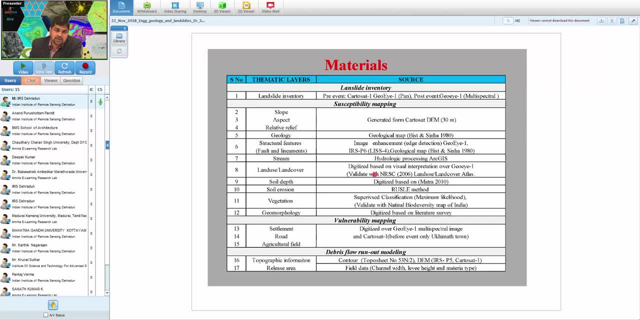 want to do a study, remote sensing on a satellite image. I want to do a landslide study. I have to start start with making an inventory. so what that inventory is? so different polygons, I suppose I take a cartosat-1 image or GI image or spot image, that is. 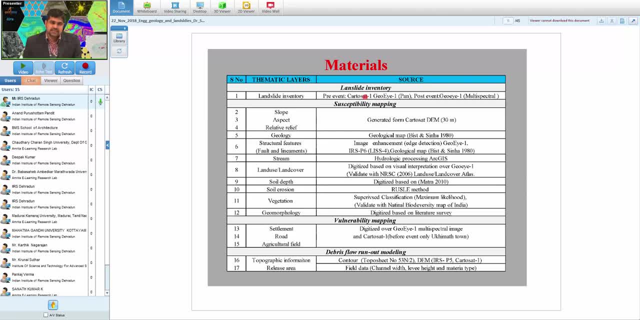 available on Google art, suppose, or we can purchase satellite images like cartosat, like LISP4, and see where my landslides are present. so I make polygons on them so that layer GIS layer will be called landslide inventory, and so inventory map rather. so it can be done using any any image processing. 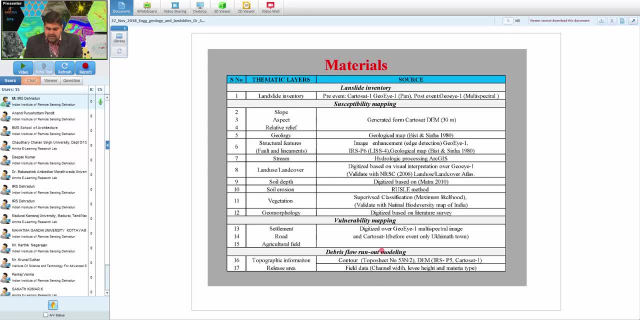 software, mostly ArcGIS, like that. next, if we come to the vulnerability mapping, vulnerability mapping we have to understand what vulnerability is. vulnerability is element specific. so what does it mean? suppose vulnerability of an area will be is a factor of the population present there? the roads are there or no, the capital states are there or no, agricultural croplands are there or no. so these are. 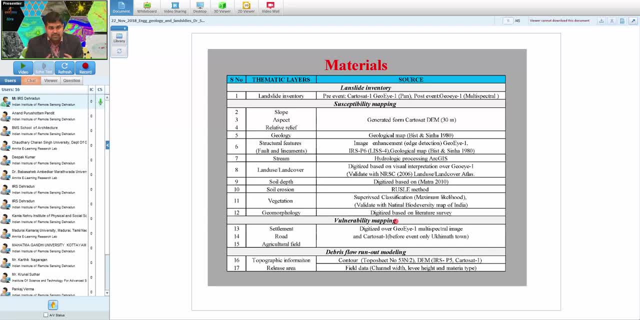 elements that are put at stake, so then becomes vulnerable. so vulnerability analysis has to include all these three post layers that we have discussed here. here we have taken settlements, road and agriculture load, so we make different, different layers for that. that does each of them and then weigh them if required. 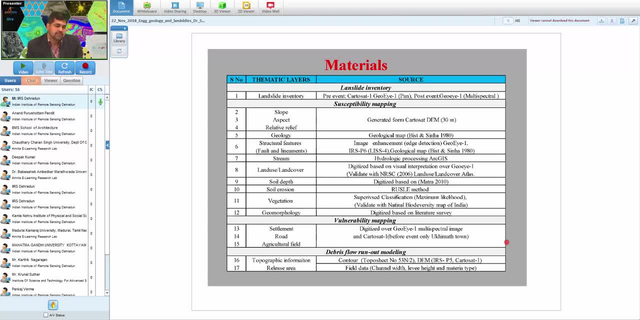 and just oppose them together. so we get a final map called vulnerability map. similarly, we get a sustainability map. it is slightly different from vulnerability, the sustainability map, if you understand the whole set of these layers- slope aspect, relative relief, geology, geophology, structure, geology, lineaments, soil depth, etc. to be taken at 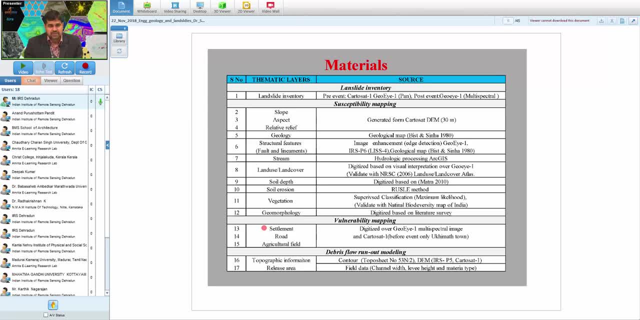 reconsidered. you may take more or you may take less, depending upon the area, the size, etc. so so sustainability basically means how much sustainable that area is suppose in terms of distance from a stream. if it is very close to a stream, there are possibilities that it the moisture. 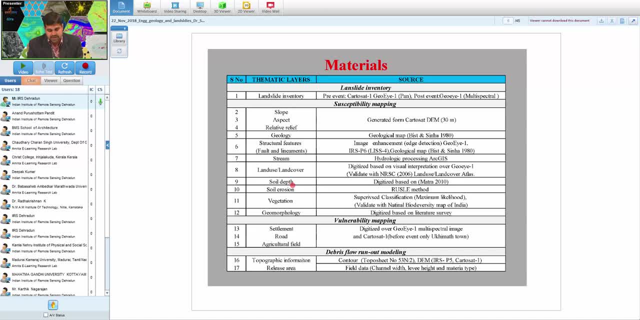 because of the moisture, the slope stability may be hampered, may get hampered. or suppose it's close to a like here in there, the very close to Himalayan fault system. so that basically puts this makes this area sustainable because of the proximity to the MBT or MFT, MCT like that. so it's seismically. 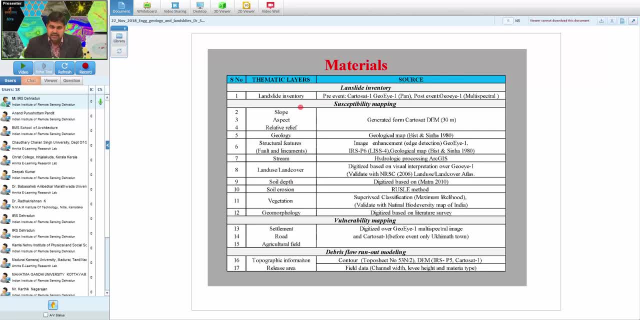 active those thrust and that makes the whole area unstable, like that, if it happens on a sufficient slope, suppose. so the whole whole thing becomes unstable. so these are the layers that we need to consider for calc on sustainability mapping. so once we get sustainability mapping, we get vulnerability mapping. we 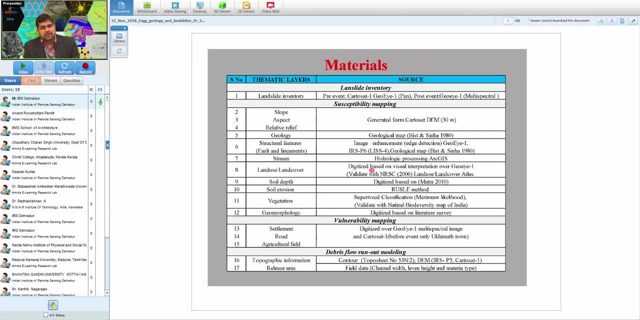 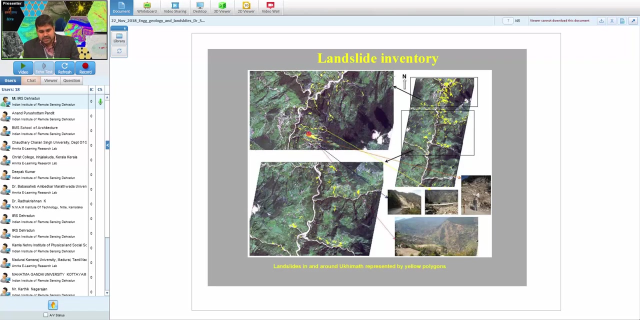 can put this together. a cross product of that often is what we call risk, risk of an area. another last part we will do using a software called RAM, so that will learn here. basically it can cater to the mitigation directly. this is what I was talking about, the inventory part. so inventory is nothing. 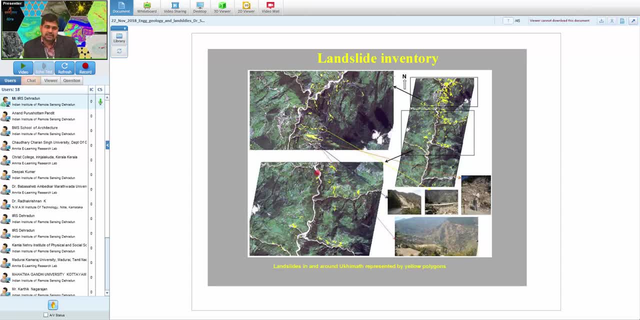 but can you see the polygons here? yellow polygons indicate that there are landslides. here we go about. the world law of zero is the present, is the key to the path. so that basically indicates that if something has happened, reverse ways. if something has happened in past, landslides happened here. that 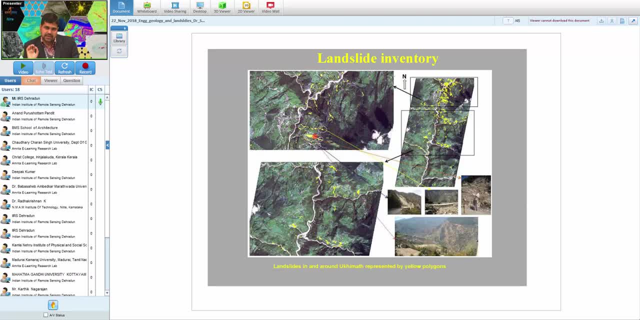 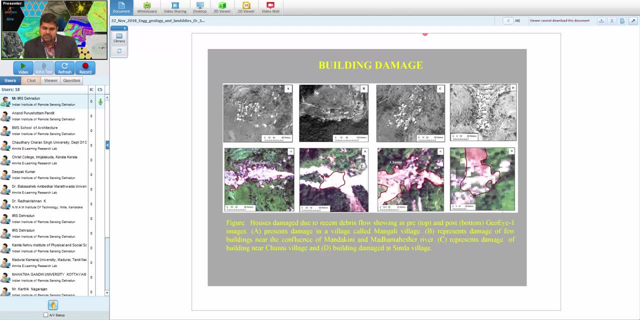 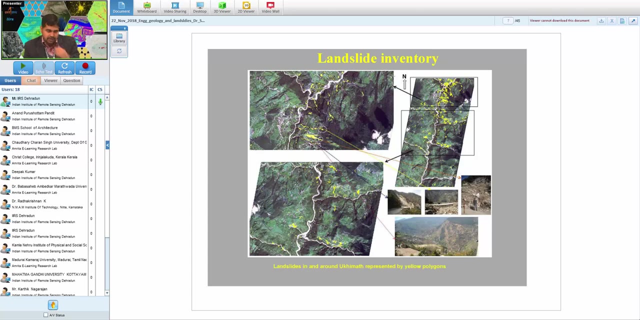 area is important or a landslide, that area becomes landslide prone even today. so that is why important now how to use this inventory layer. so first we start with the inventory layer, like this: j on gis, we get a, get a safe file or a factored map, i'm sorry, a thematic layer of landslide. 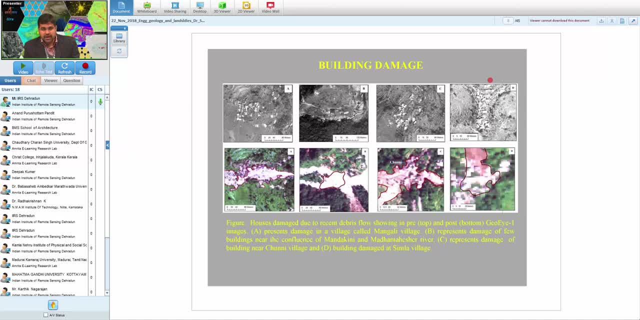 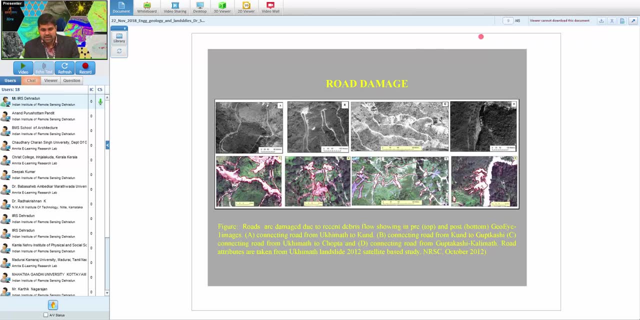 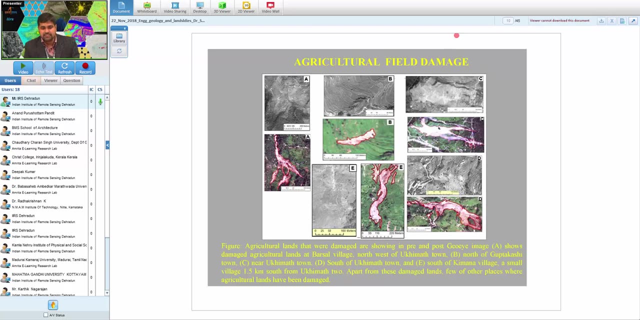 inventories next week up to onto the vulnerability analysis. for vulnerability i have taken building damage here. which are the buildings that will get? may get damaged, road damage, and suppose we get agricultural field damage. so which are the area that may get devastated if a landslide happens or something has already happened, post facto and before the landslide happens? both we can do so. 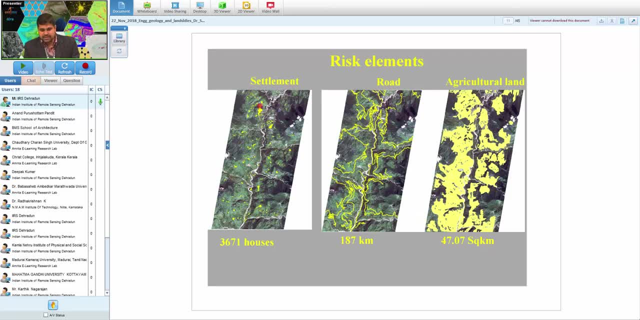 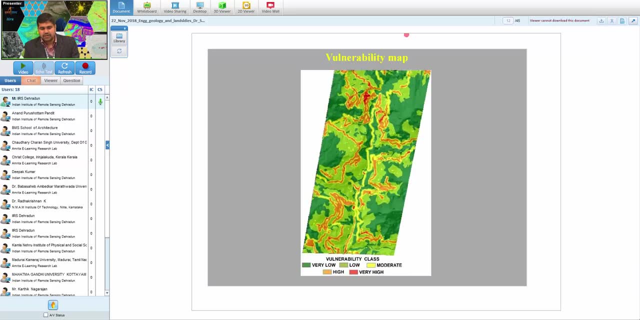 putting these three last three layers together, so settlement. let's see, these are the settlements, these are the roads and this is the agricultural land. if i put these three layers, i get what is called your vulnerability map. so these are the vulnerability map. please see, we have classified. 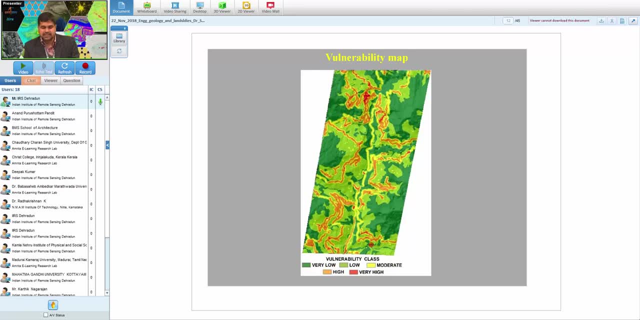 again from very low to very high. so five classes, so very low to very high. obviously this road- because we have put some weights on this road- is an element that is very vulnerable. so that is why all red you can see along the roads only so we get a. 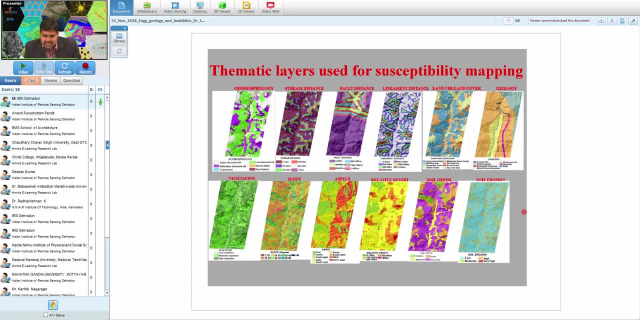 vulnerability map like this for susceptibility mapping. we take these, suppose, 12 layers here: geophology, stream, distance, fall, distance, geology, slow prospect. if i put this together, there are different methods involved, how to do that. i'm not going to show you how to do that, but i'm going to. 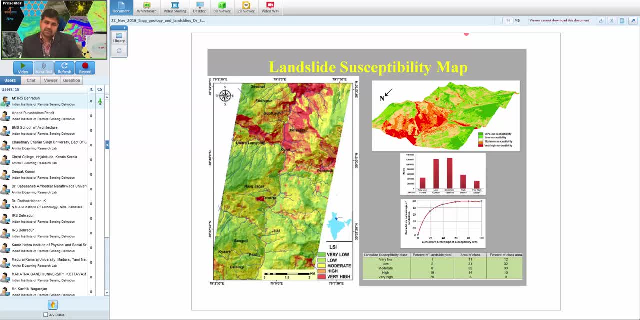 do that. i'm not going to show you how to do that. i'm not going to show you how to do that, i'm not going to in detail about that. but there are some knowledge based methods, there are statistical methods. so these, by doing any of these, depending upon how your area is, you can get a sustainability mapping. 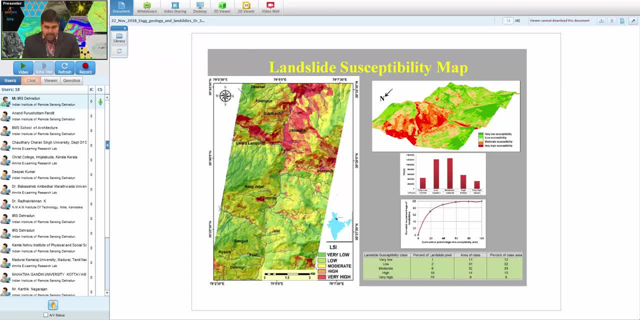 so it's just basically putting those together and getting a map using different algorithms. so, please see, this is called sustainability map and accessibility. again, the map has been reclassified in from very low to very high classes. these are the areas. red areas will indicate that it is. 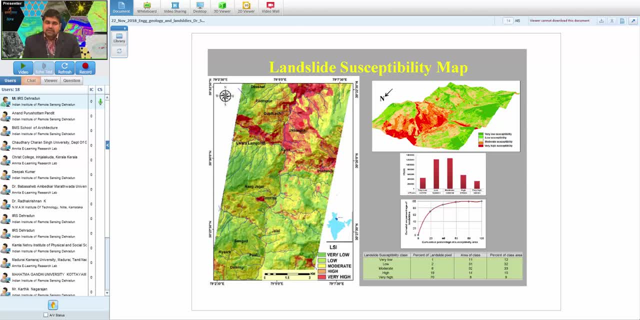 very much sustainable for a landslide people. quite often they stop at doing sustainability mapping only and they make this equal to a hazard map. so i mean in a loose sense we can call the hazard as a stability, but beyond that we can go for calculation of risk also. so for that risk we need 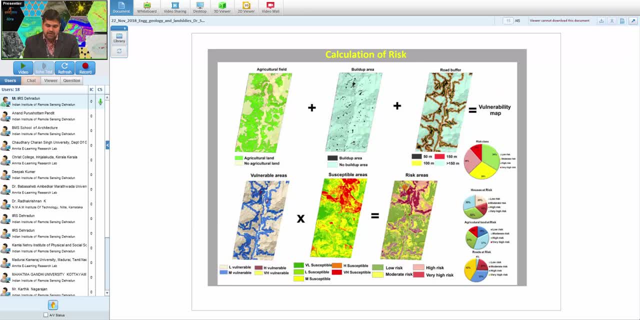 a vulnerability map and the sustainability both. if i cross it i get a risk map. so that is my ultimate pro dot. but again, you have to. you have to understand that high risk areas: how do, how do you validate this result? this is the area which shows your uh four support risk zones and very high area has to 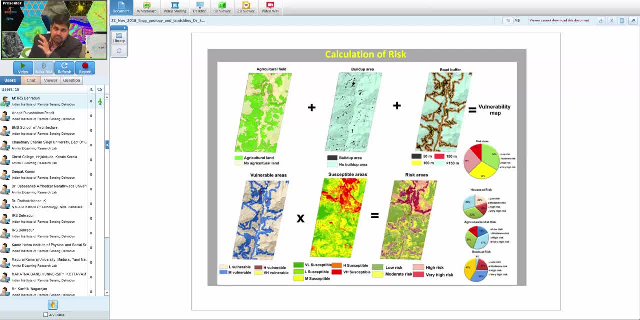 it has in the area is supposed to contain maximum more of your um the polygons where landslide you have marked on inventory. so if you juxtapose that inventory layer on your uh, this risk layer- high risk- should contain more of the landslide polygons if the landslide polygons are falling. 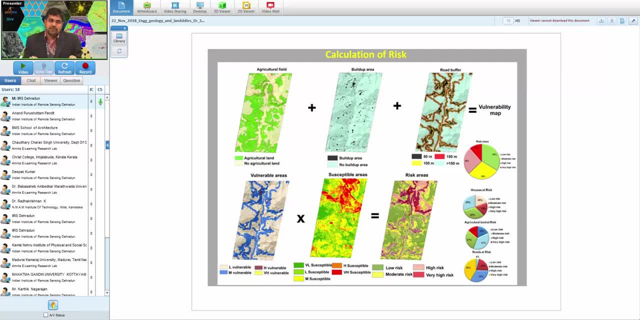 somewhere else. that indicates that somewhere something. uh, we have made a mistake in gis. maybe the proper thematic layers for sustainability have not considered, maybe we have considered more layers so that my original uh influencing factor has got somehow diluted, or maybe i have taken, i missed the main layer. this is also possible. another set of error may come from. 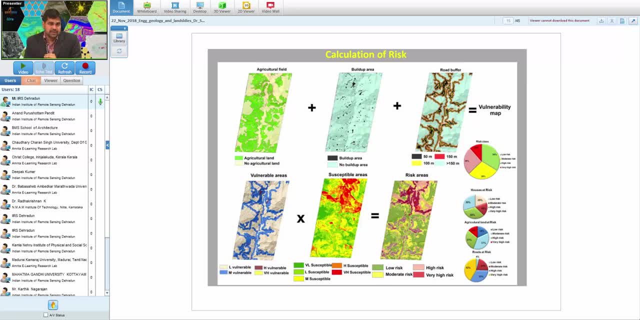 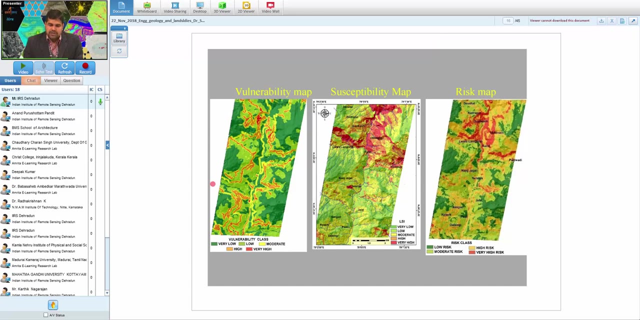 uh, the method that you are applying. so this is the mathematics part behind this. so, but in most cases, if you have done all correct, then your landslide polygons will fall directly up above your high risk zones. so if i put this together side by side, i can check vulnerability map. 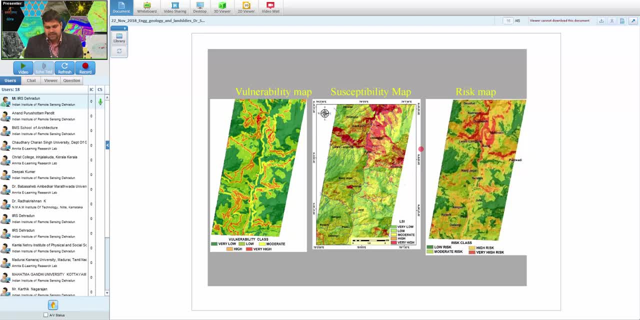 sustainability map and risk map. you can check where the risk is more, but vulnerability map is more of a risk and risk is less and risk is less and risk is less, but vulnerability map is more of a risk and risk is less and risk is more of a risk and risk is less and risk is less. i will give you two. 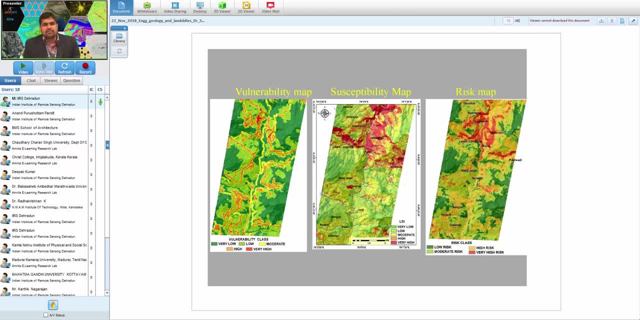 examples. suppose i'm on to ladakh, somewhere in ladakh where you know, very less building, popular, very less population. uh, there are not much building infrastructure. roads are also quite less in number in frequency, so the vulnerability elements are missing. so that makes the vulnerability very low, but at the same time the area is very close to uh himalayan fault system seismically. 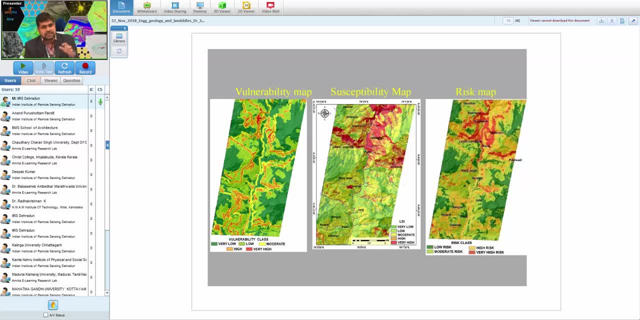 very active, so that makes that area very much unstable. so if i cross this low vulnerability I get a low risk again. suppose I take you to a flat land, suppose a city like Kolkata, where your it's highly populated infrastructure is very developed, so all vulnerable elements are there. but 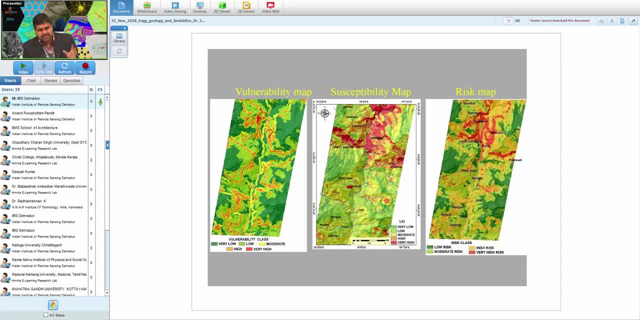 again, there cannot be a seismic that not much affected by seismic events, and you know so that makes this area very low in susceptibility. so high vulnerability, low susceptibility again gets my risk low. so there is a zero hundred, this variation from zero hundred to hundred, zero in between. 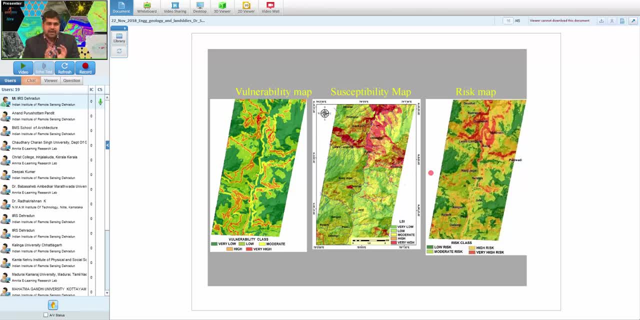 mostly we have all my risk maps calculated. so we will not generally have either this end where hundred zero or the zero hundred but in between a value will get. so let me clear to you one thing: that this risk map calculation we should not stop at that, that the risk has covered all aspect. it. 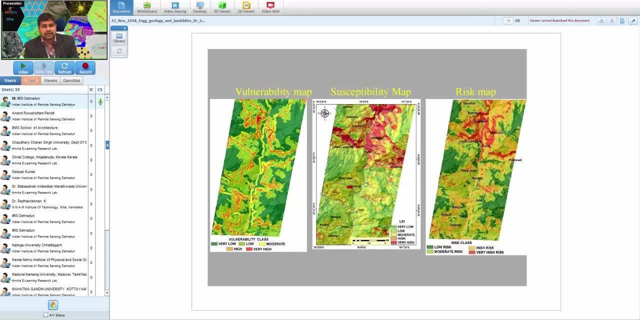 has come, but it's a fact. factor of vulnerability has to be to have seen. but what beyond that? there is another factor called factor of safety. the factor of safety is a major feature. suppose an area is vulnerable and sensible, both. but the area contest, the buildings will, who are very well reinforced. 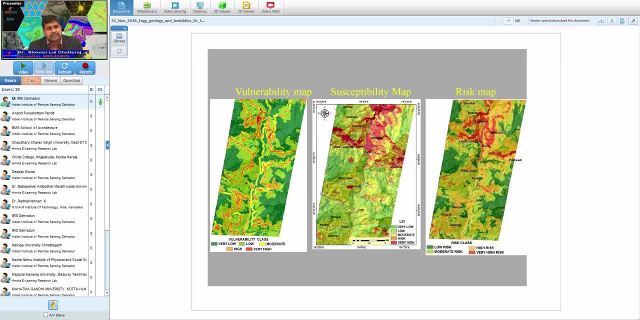 has used very well reinforced concrete art for earthquake resistant structures are there, so that makes the area strong, that makes the building strong. so factor of safety is to consider if vulnerability, susceptibility and factor of safety- these three together can be used for calculation of risk. but risk doesn't encompass only these three. there's another factor: the exposure. 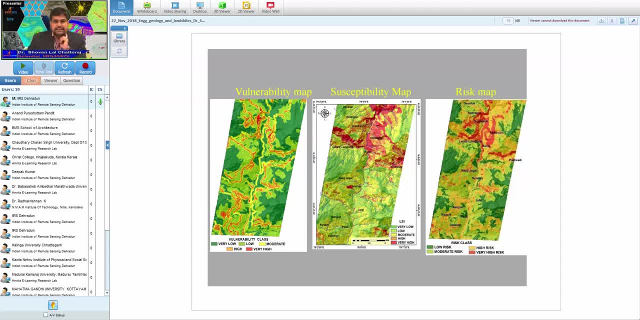 the demography, suppose which type of people are exposed. the area where i'm calculating this, i'm determining the race mostly concept, has a concentration of, suppose, tribal area. so obviously the risk is more. or some area where risk, where, where the demography is such that it can easily sustain to any kind of 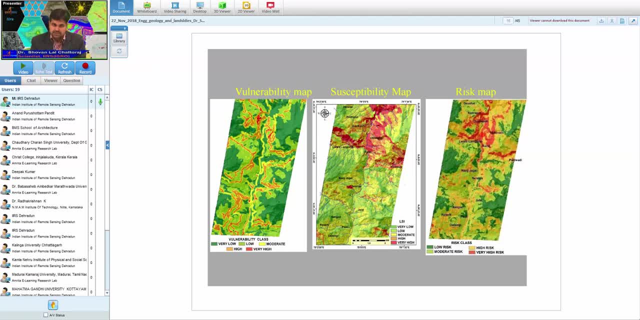 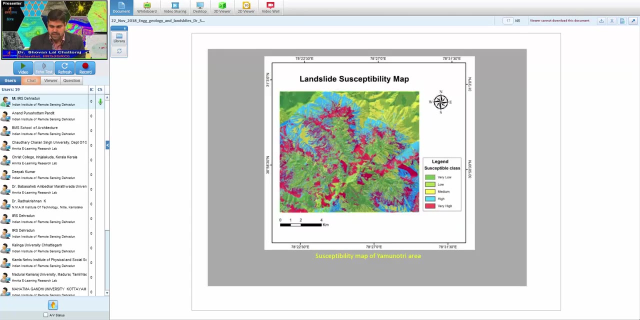 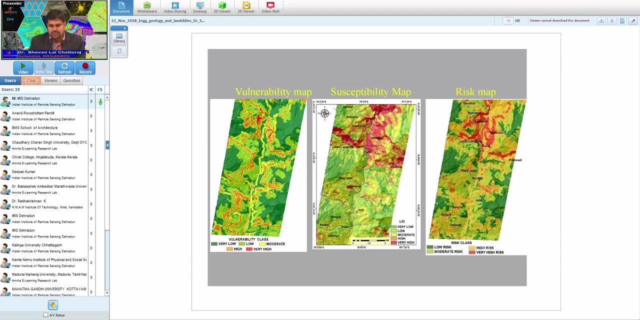 disaster. so that makes the exposure basically will control the risk of that area. so risk by now we have seen that you know, considers is a factor of rather vulnerability, sensitivity, factor of safety and the exposure. we have similarly calculated risk zones from this. this risk map was from northern part of, I mean, I mean in in. 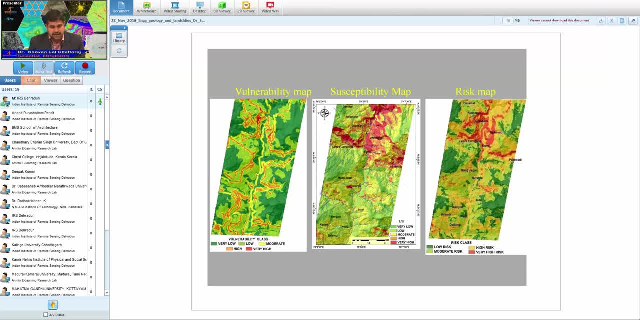 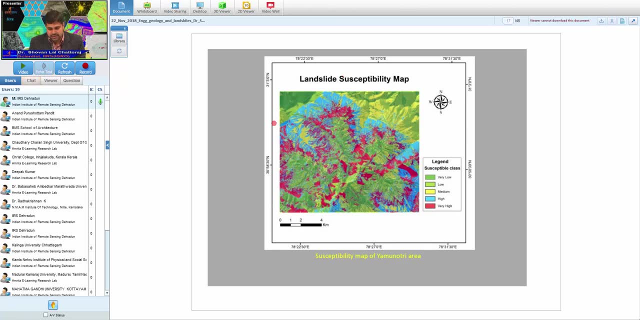 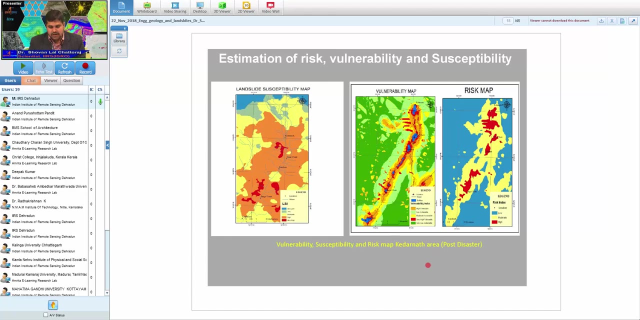 Rudraprat district close to Kedarnath area. this is from Jamunotri area. we have calculated post Kedarnath yesterday, have calculated this hostility map of that area at this scale. we have got five classes out of that. similarly, the post Kedarnath event in the same Kedarnath Valley area tried to calculate the risk. 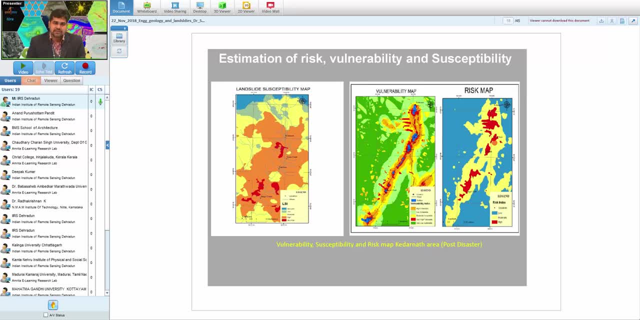 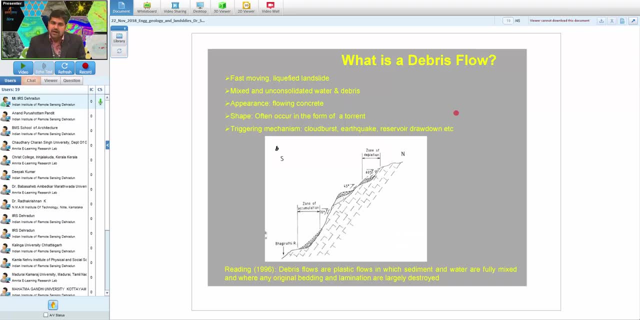 and we have seen that most of the areas which were devastated, they were lying in very high risk zone. now we come to the modeling part. so here, mostly, we will try to model a flow flow, event flow type of landslide that is called debris flow. what they are? they are basically liquefied, fast-moving landslide. they are: 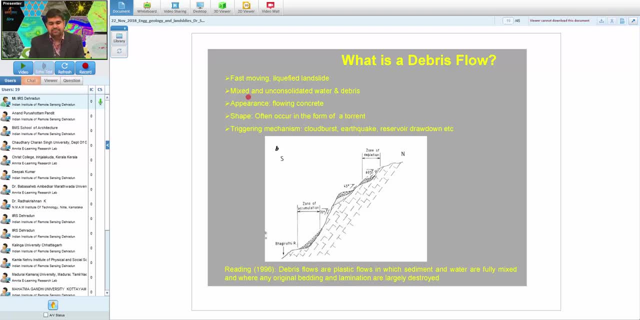 mixed with the flow of the landslides. they are mixed with the flow of the landslides. the appearance is like a concrete, and then they have. they will often flow in the form of a terrain torrent. the triggering mechanism can be cloudburst, can be earthquake, can be reservoir drawdown, anything so this zone will be. 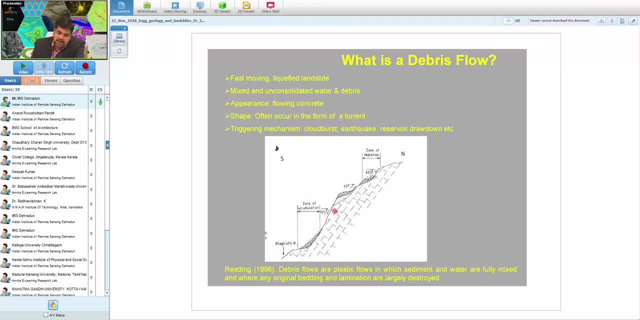 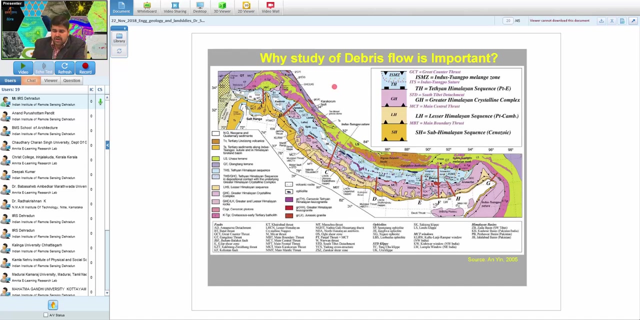 called zone of depletion, the source area where from material is going down and this is the zone of transportation and this is the zone of accumulation, where you get your debris material accumulated, deposited there. why the debris flow are important to study because you know where we're currently standing. we're very close to the proximity of Himalayan fault systems. 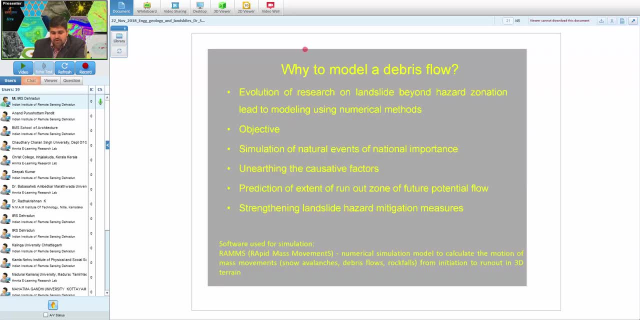 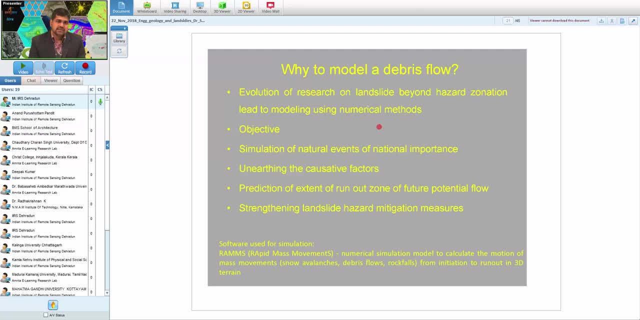 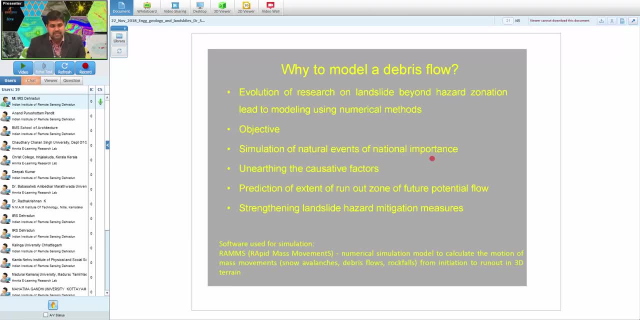 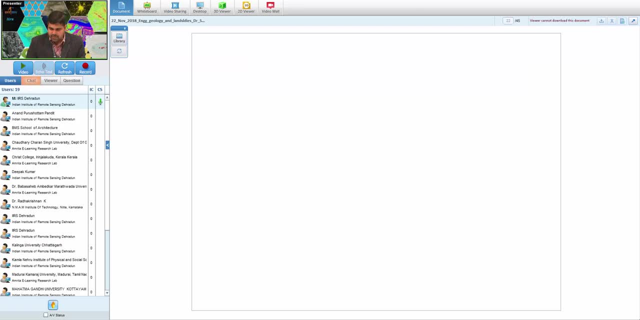 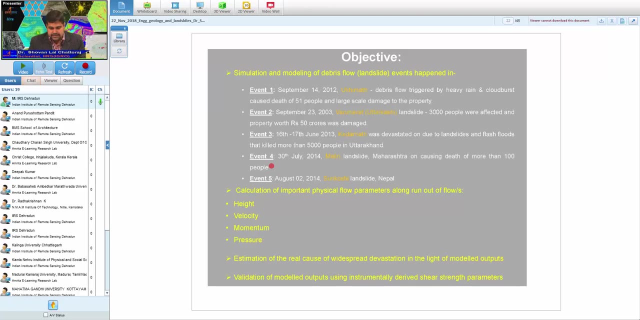 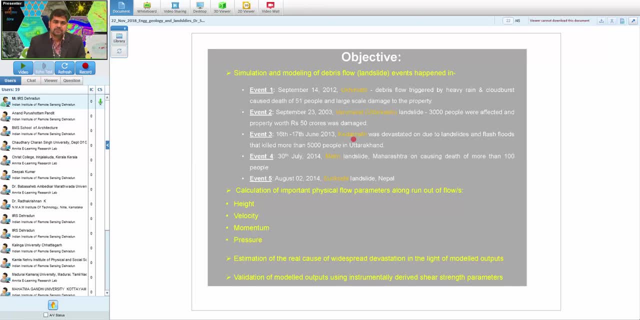 was the famous Kedarnath one that happened in June 2013, and then Malin landslide, because we wanted to see whether our model works well using works well if we are outside the Himalayan zone. so that basically took us to the Sahadra Hills in Western Ghats, where we have seen the land, the debris. 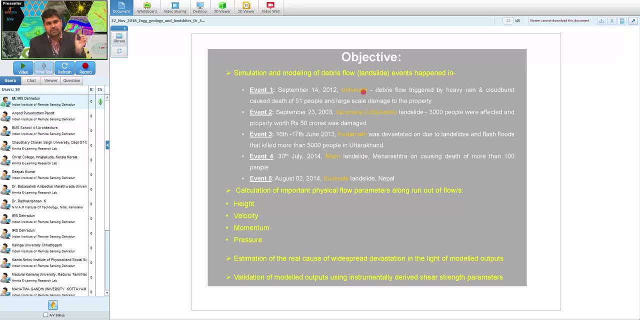 flow to be more. to get model, we tried another from Sankoshi landslide in Nepal. so what that is the Sankoshi landslide is. again, it takes its name from the Koshi river. Koshi river basically takes its name from this. so there's a if something. 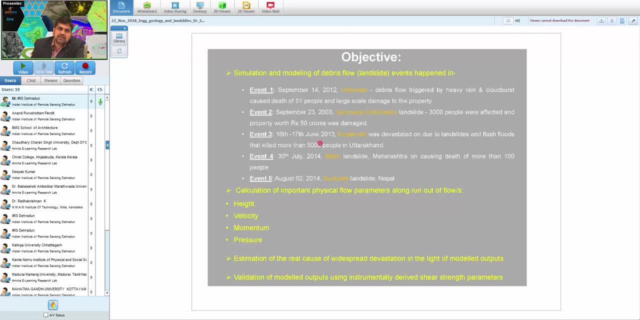 happens in that landslide, the whole Koshi river will get affected. so that happened in 2014. basically, the cal. what are the physical parameters that the software will get you to? it will calculate the height, the velocity, the momentum and the pressure- these four parameters. so, all along your debris flow, any point you can, if you. 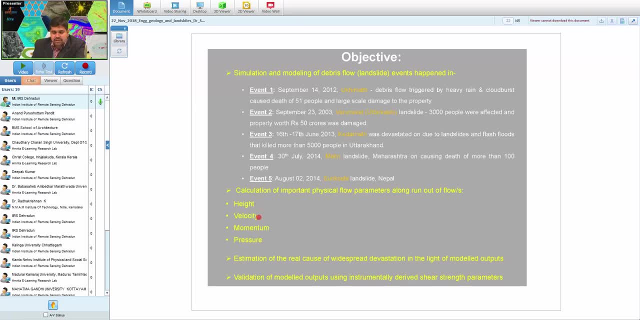 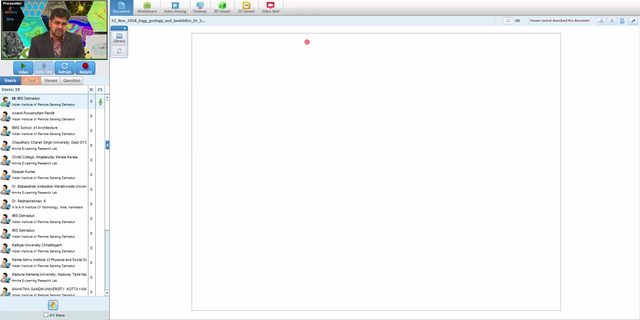 stick to so on that point, you will get to know what is the height in meters, the velocity in meter per centimeter, meter per second, and then momentum and pressure. what are the how they are very heading all along. yeah, yeah, so that is the. this is the landslide that happened in okay material. 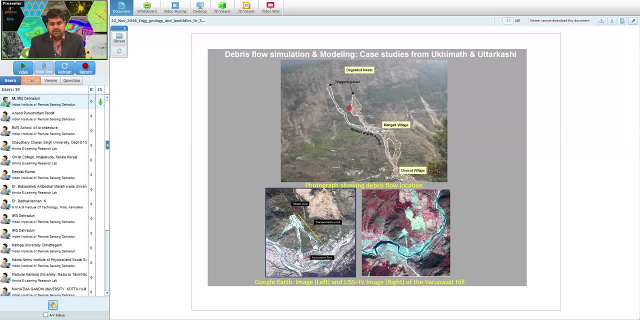 have given an example from this. so the where there are two villages to villages, where there is one monthly village, one Chimney village was there. these are the source areas. well, from the material were dragged down and there's River flows here, so it get deposited there down, down slope. now the Bernabas landslide, as I've 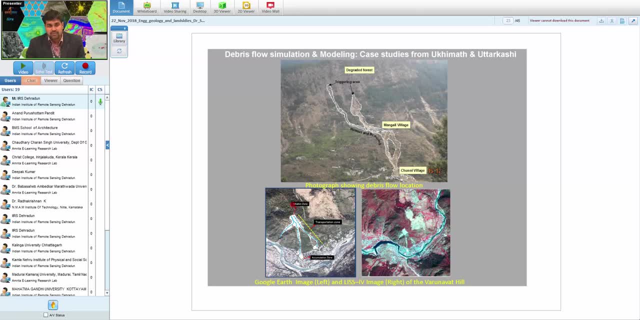 told there's no life-losses and there's no other side, and then you will see an as such, but the huge property loss was there. so there is a type vacation of landslide is a typical case where you can model using your landslide, using your numerical simulation. so there is a type vacation of the flow. so there is a. 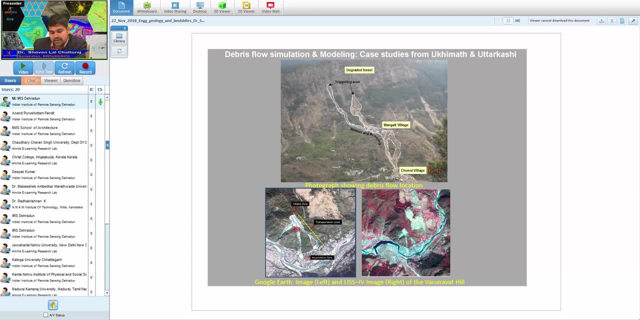 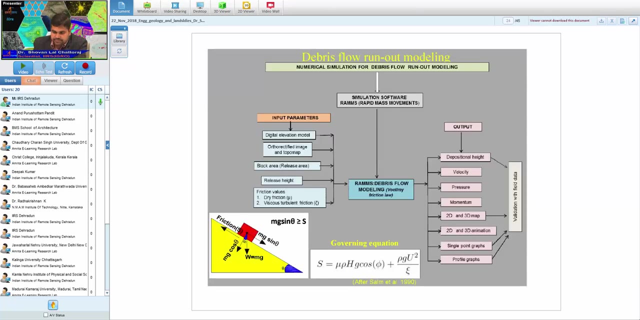 type vacation of flow with the source area burn about the landslide and the flow. there is a type vacation it reached. when it reached there, it deposited a lot many buildings. in satellite image it will look like this: this is the source area and you can see three legs of it. so this is how the model walks. so we have 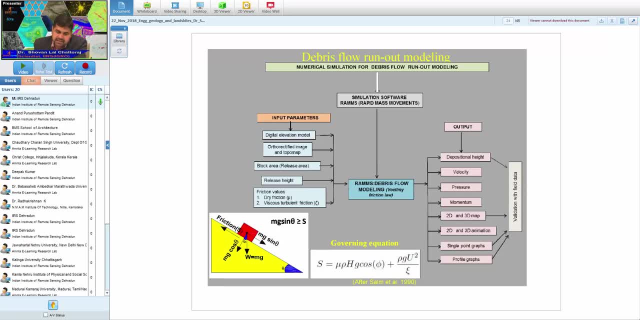 to understand what is the mechanism and is the algorithm part. so this is the very part is supposed by the material that is, it's hanging there, it has to go down. so the empty: it's hanging there, it has to go down. so the mg is the weight. so if the theta is this slope, then mg sine theta is the force that will uh, that will uh make. 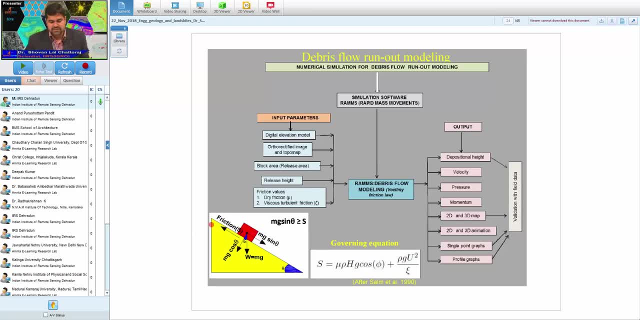 it flow down, obviously being opposed by the frictional forces. the picture forces, suppose is capital s, so capital s. it has two uh portions. so this portion, which is a debris flow, so it will consist more mainly of rock chunks and your water, so the rock chunks will have its separate. 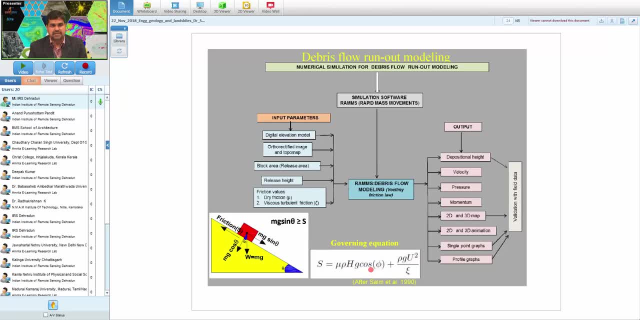 coefficient of friction. water or any across medium will have its separate its own uh frictional coefficient. so that is where the friction from both these phases will be different. so this is because of the solid phases, the friction due to solid pages. this is because the friction due to 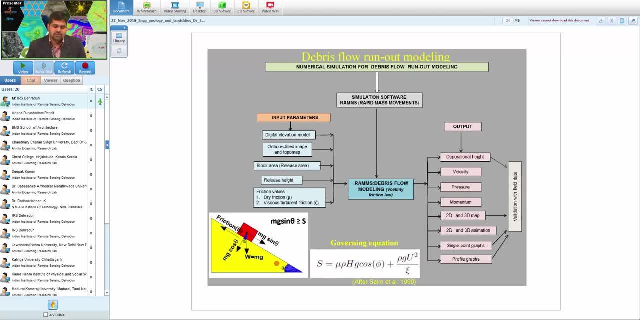 the liquid phases. so if i put that together i get my total friction. so once the governing equation is that once my ng sine theta- this is the gravitational force- is more than equal to total s, uh, it will start flowing, it has. it doesn't have to be always more than s, even if it is equal. 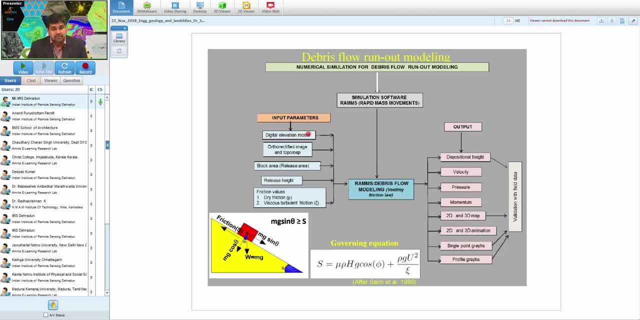 the flow, the slide will start. so for input parameters you have to give a very good resolution dm. maybe less than 10 meter if possible, and then on that dm will delineate the source area very clear. clearly you have to get the source area. so once you give a source area on, 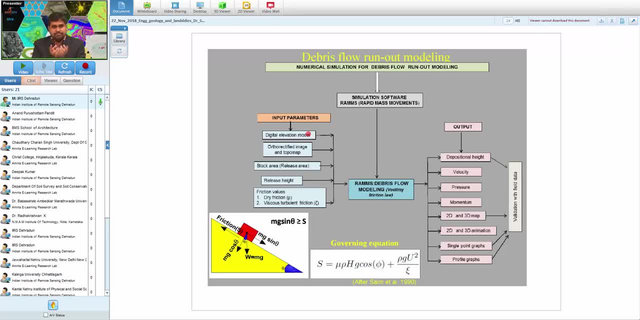 a very good resolution, dm. we need to understand what is happening. basically the, the amount of the. this is the volume it, the software calculates. so any dm will give you a topography, very good topography, topographical variation, and if i draw a source on that, that gives me x, y and all points. 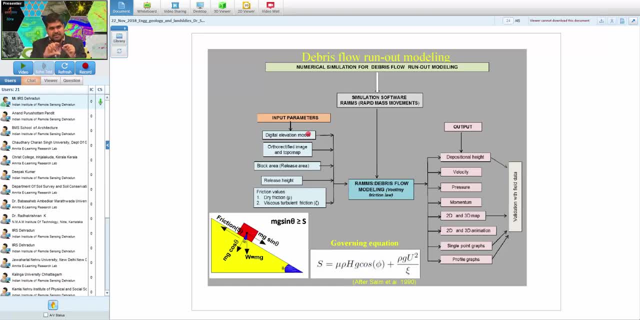 of this, x, y will calculate from all points. when it reaches the base we'll calculate the z's. there's the depth, so all z's accommodated, it will give me total volume. so what the software does is basically it. it gives you clues about how much material it is flowing with. so there's the volume, basically. 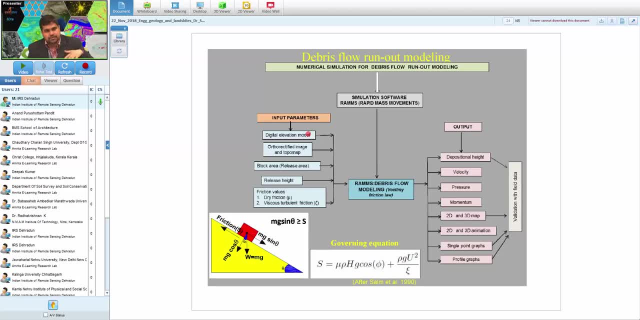 next. number two is where it is flowing. so on which slope, suppose. so dm again, uh, gets me a clue about that, on how much slope it is flowing. and third is with what type of material it is flowing with. so what type of material means the frictional coefficient? that is, a granitic material or marble? 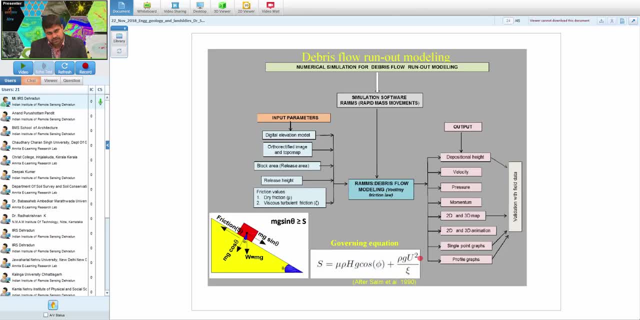 or loose clay sediment- that is, a granitic material, or marble, or loose clay sediment. what type of? how much of water is there if the water is completely muddy? so the friction parameters will vary and accordingly this rule. so that gets me various models. the output parameters, if i look into will be a 3d simulation. along with that we'll get profiles, 2d profiles, additionally. 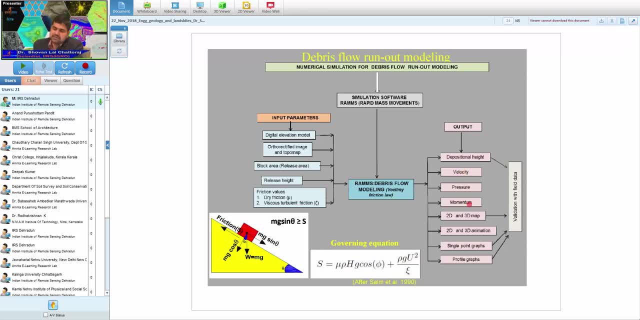 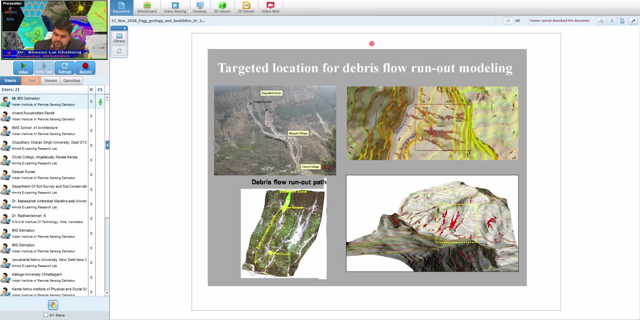 any point. if you click on that model, your model, you can get the velocity, pressure, momentum and high us, even if you just type it in description box. so if you just input this in the description box and then you go back to the tool, is because the control panel will hold all the relationship. 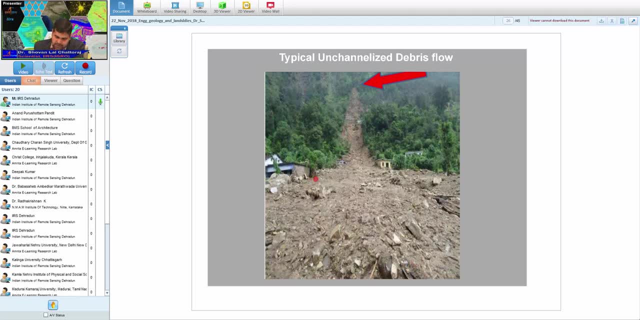 data. so if I click on this, whatever is the shocking value, i actually music is pretend to phone to him. so you have to connect it to my go account. so the control panel is just directly connected to the spam data. so at that point i cannot connect with the go address, but the control panel will. 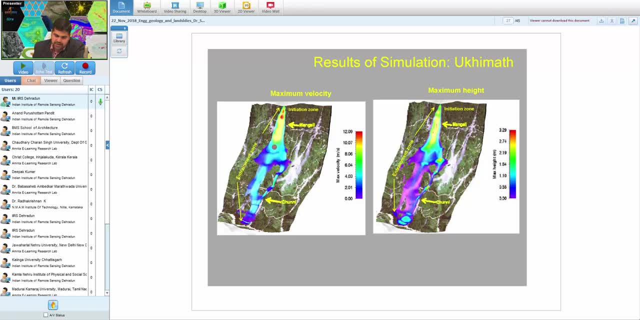 just know my to go and connect with the go address, then the control panel takes you to a Command depicts. so this is what the result will look like. so, any point, if you click according to the scale here, we get the velocity. suppose this is the road. if you can identify this is the road, 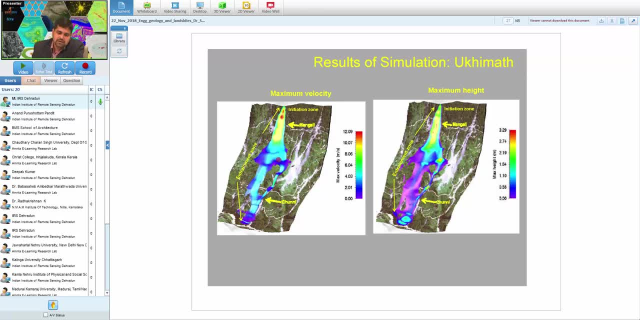 and here it quite. it happens quite often that single road, you know it goes like this, a fashion like this. so if landslide happens from hill, from higher elevation, the same landslide will cross cut the same road many times. so you will get blockades here, here, here, here, same landslide. 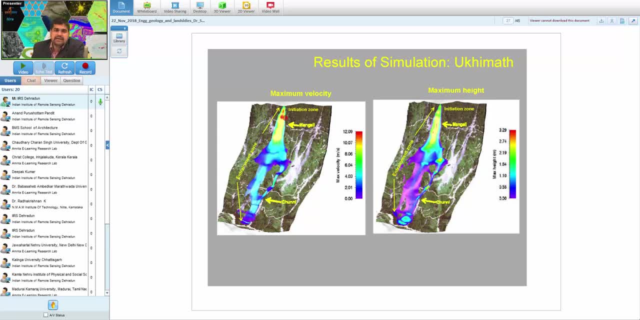 now, if i, today, suppose tomorrow, if i, the landslide has happened and next, any season onto, some more material is going to come to erase the flow, if i want to take a remedial measures, what do i take it here? i can construct a dam kind of thing, so that wall, so that you know. 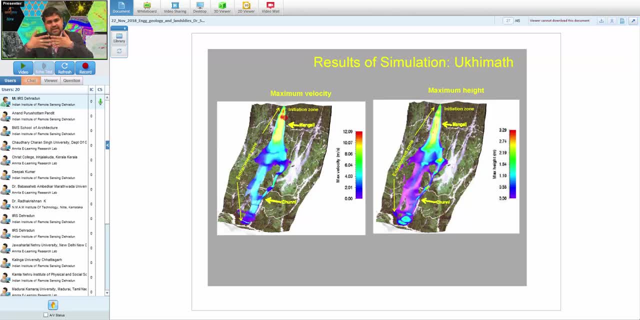 from the slope. if something comes, it will get deposited on the other side, over the other side of the road, so i can construct a dam, so that wall, so that you know the wall now it will not come onto the road, so my road doesn't get blocked. so there's the idea. 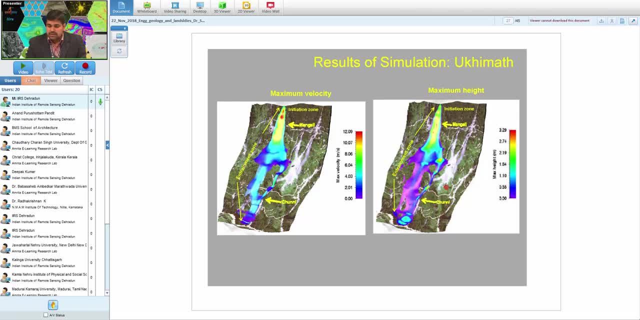 but what should be the height of the dam? the height of the dam, the idea we can get it from here, what is the height that is expected because of the debris that is coming? we can calculate from this: suppose three meter, 3.5 meter. obviously my dam has to be more than this 3.5 meter height. 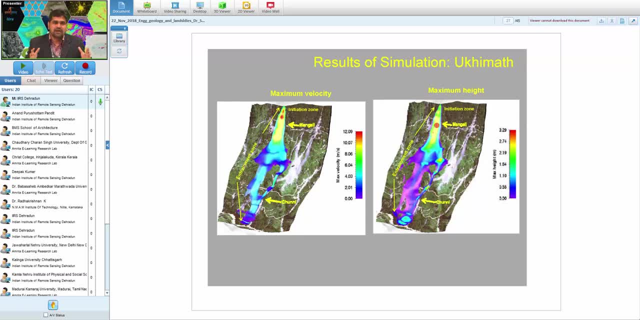 it's not about the height. always suppose some. you know big rock chunks is coming and you know it's a high momentum. now i have made sufficiently high wall to arrest, to digest the initial flow. but what about the width of this wall? the width has to be sufficient so that it can withstand. 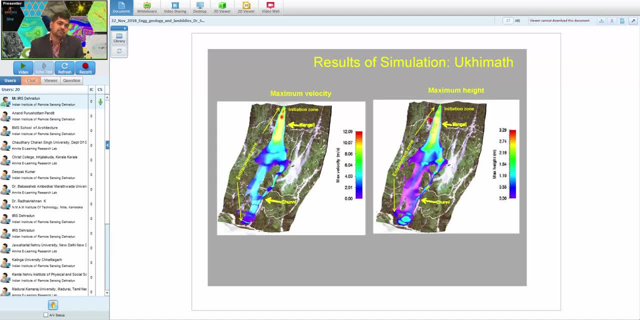 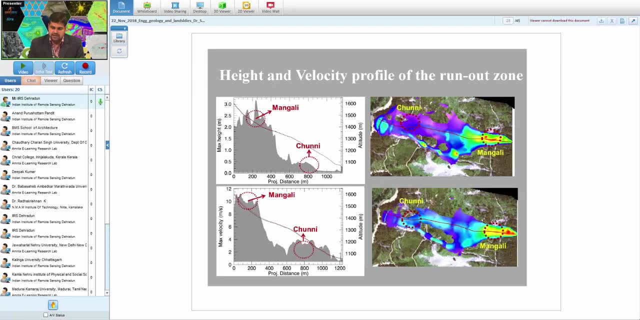 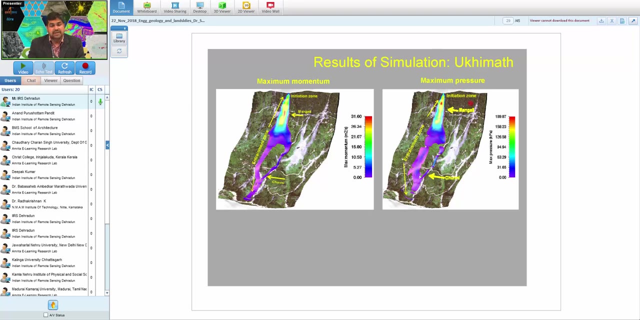 the flow, the momentum. basically, if it doesn't, if it cannot withstand the momentum, it will be broken. so that is why the momentum is also required. so here is what we get: the height and velocity. along with that that we get the momentum and the pressure. so all along, I can get. 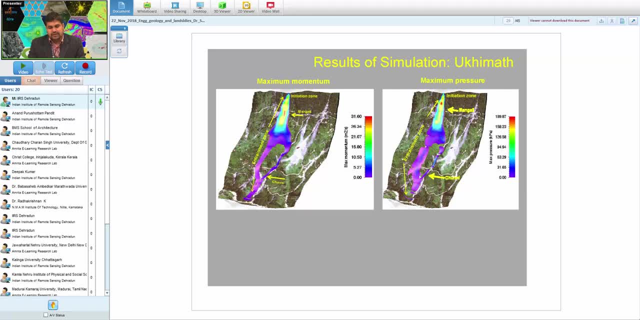 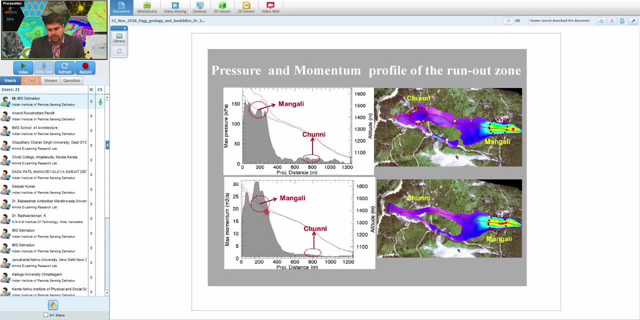 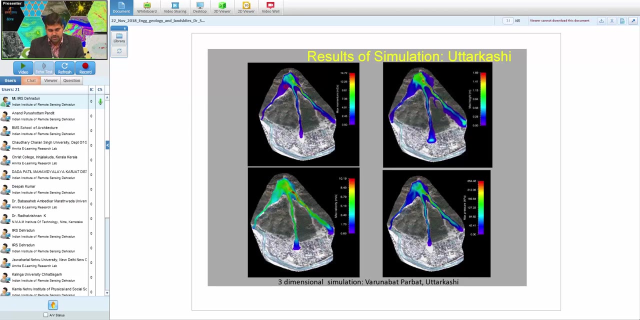 all under the entrainment path of transportation zone, I get the momentum, variation of momentum. so any point you click, you will get it. or on a profile also, you can see it like this: same result we have. I have shown you the example of Uttarkasi, where trifurcation has happened. similar results, we get it. 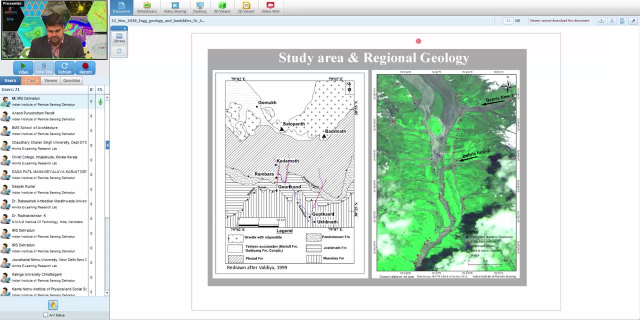 from here again the profiles, the cadernath one. I got tried, so this is work you're creating. a term is a list for image. this is where you cannot temple exists and this is a major debris flow. there is a feeling that every where that okay, that a together, not these two- happened, happened mainly because of the 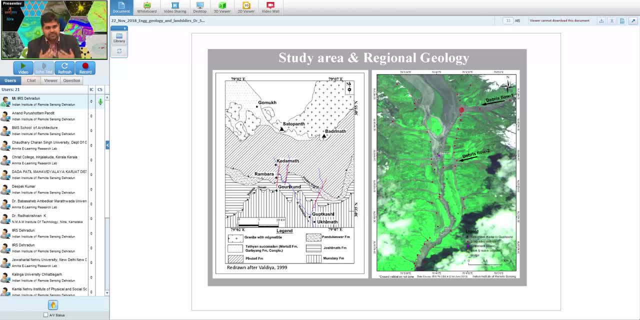 so much of water that became available into this narrow valley so that everything got washed away back to where we have seen. that water available to that was not a not that much quantity, that much of volume, so that devastation of this kind it will allow. we, using our satellite data we have published to this 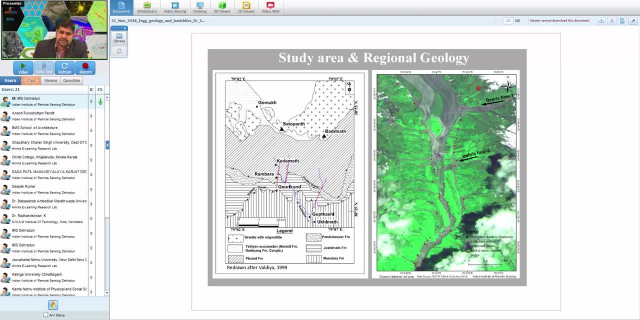 work in natural hazards journal also, if you are interested, you can have a look at it. we proved that there are the debris flow that basically brought its material and got deposited here. so the river River Saraswati, suppose Mandakini, was flowing like this and that took another path. that took another part. 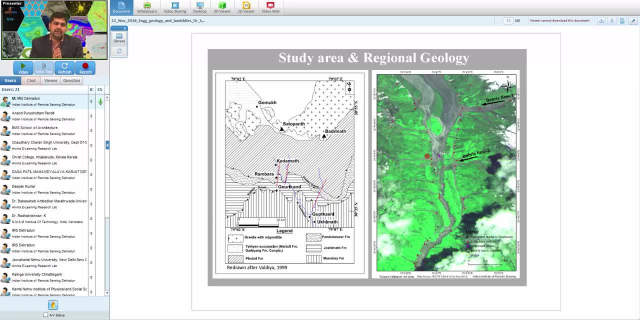 which was abandoned long before. it was a valley channel, basically old value channel that used to flow where the camera temple right now exists. so because of the blockade by the debris brought in by the debris flows. so there's a one kind of sufficient blockade development and the water had to take the least recent path, so it had to take the whole. 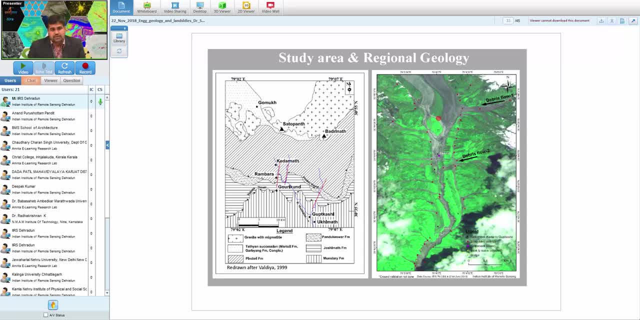 valley channel path and that is how it has to pass through your temple and town areas, otherwise you would have could have this: that much volume of water would have easily passed though this already existing existing stream path. so didn't happen and it had to take a path to cross, cutting your town itself. 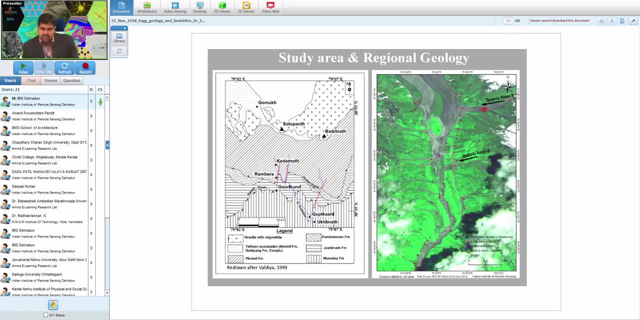 so that is why the devastation became that big here. so I tried to model this flow also just to see, just to check how much amount of debris is available to debris flow 1, how much material it can bring down. debris flow 2 occurs slightly downstream of that. similarly, we get you know a blockade here also and show the. 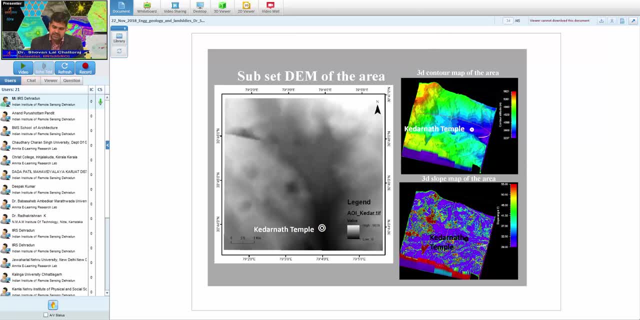 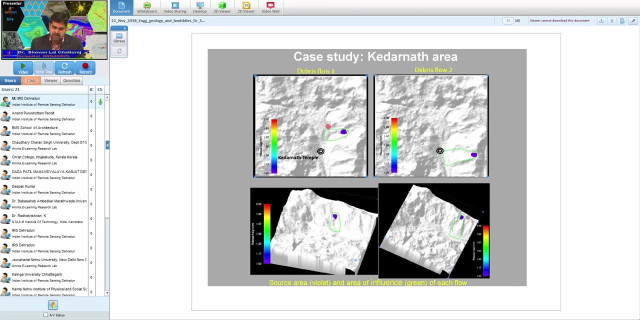 results. so this is the DEM will look like and the Kedana temple exists here. these are the source area, the source that I told you that this is the DEM and on which I get a source here. this is allowed to flow from this and, if you see, 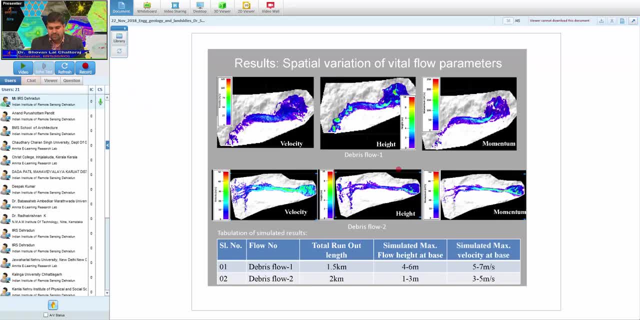 the results. it will look like this: so the velocity, the height and the momentum for both the flows has happened like this and see the maximum velocity. maximum velocity at base. maximum height: 6 meter height. maximum 6 meter height of debris, the debris flow. one could have brought a rather 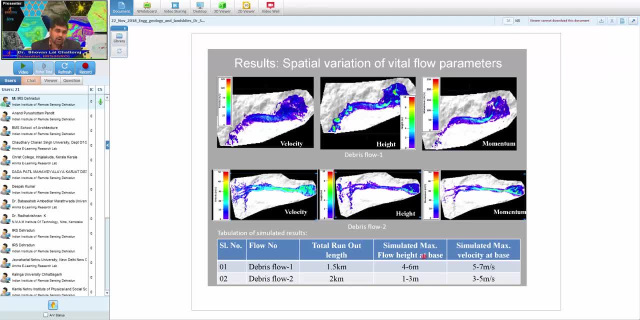 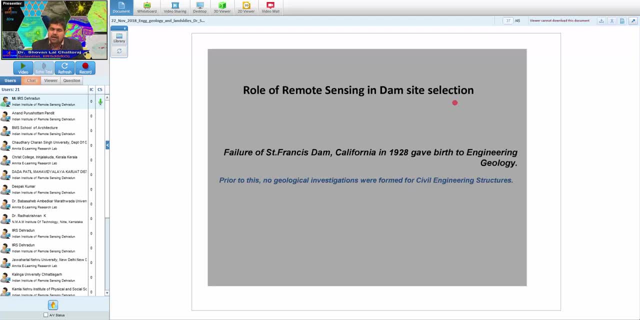 wouldn't have brought a lot of debris, but it would have brought a lot of debris, would have brought into this stream, so that it got blocked and the river had to take another path, another rather unusual path now I'll come to. once that is over, I'll come to the dam selection, because the lecture was about engineering. 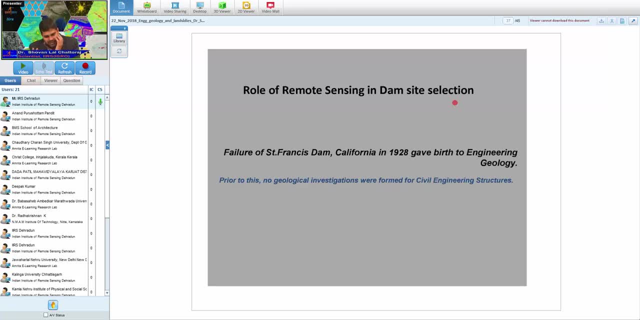 geology focus on landslide. so landslide part we have already covered. I'll spend a little bit of time on the dam site selection. that is also very much important if we want to know about now what help we can get from remote sensing. so they as such, the engineering. 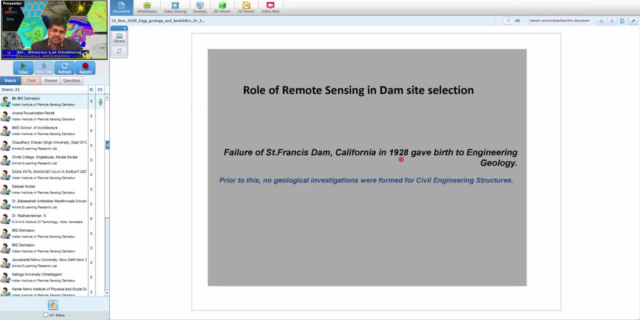 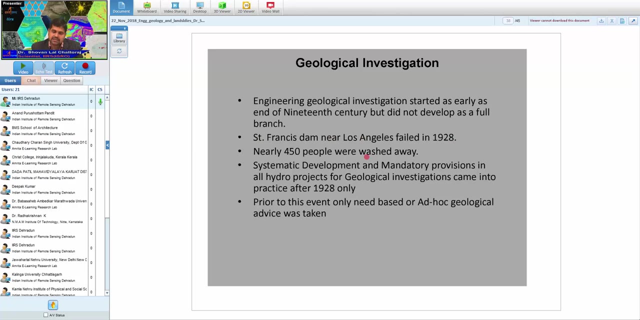 geology before 19 to 1928 doesn't and doesn't being was not being considered before the failure of this st Francis dam. that happened in California. so what are the geological in this? to st Francis dam, near Los Angeles, failed in 1924. 50 people were worst ever. so that is the. 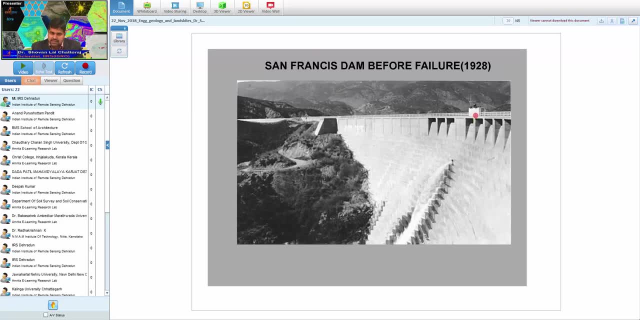 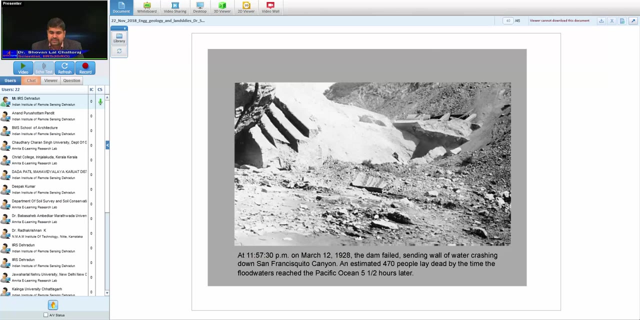 even that reminded us that engineering, geology, is a science that is to be considered before considering a dam, before implanting construction, and it is the arched dam that is that used to happen there. and then, after devastation- the at 11, 15, so the wee hours of the day- the dam failed like this: it got washed. 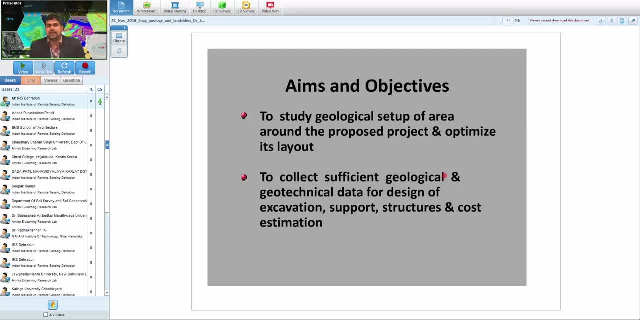 away now. what are the objectives that we are going to fulfill by using satellite data, remote sensing data? how do I get alternate sites of dams, powerhouses, etc. in a, suppose, a hydroelectric project? so the remote sensing can help in studying the geological setup of the area around the 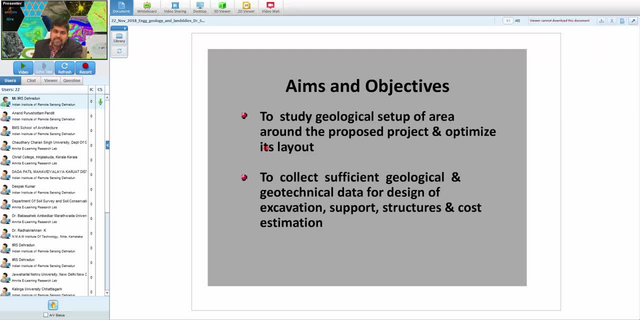 proposed position, optimize its layout so there can be three, four alternate site, but which one is the best? which two are rather the best? so who will tell that? remote sensing has plays a major part in telling this. basically, where do I need to construct a dam? we need to understand this very clearly. first is that, if it is, 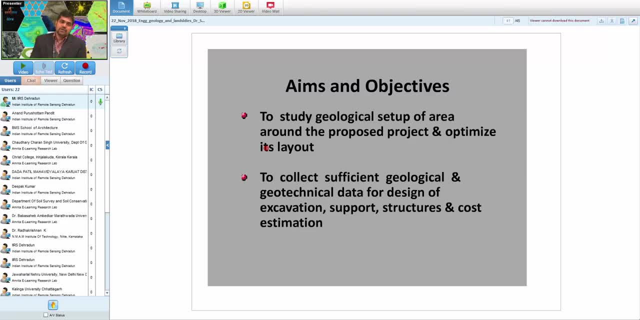 for hydroelectric power generation. sufficient water is to be maintained in the reservoir. so that basically takes me to finding an area where there are sufficient water is available. so generally, we consider a major stream is coming. it contributed to that joints into this stream. just downstream of this, just downstream of this, we are supposed to construct a dam. 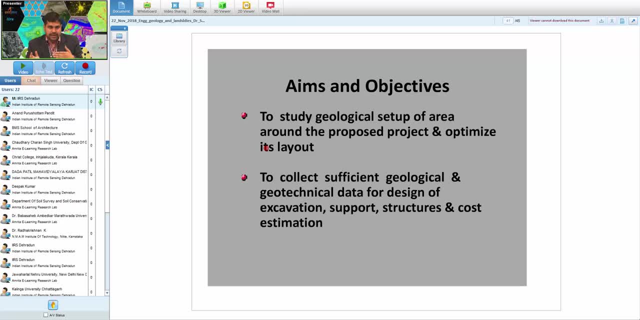 because the availability of water is big here all throughout the year. we have to search for another area for areas where the water is available and the water is available all throughout the year. we have to search for another area for areas where the value as such is narrow here, so that will involve less concrete. so the 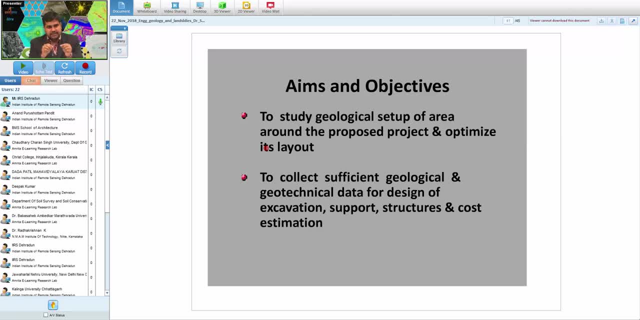 construction cost becomes quite less. so that is why the immediate downstream, of immediate confluence with the major stream and in narrow Valley, these two other factors that remote sensing can from satellite analysis of satellite image, remote sensing can tell you that what you look for this kind of areas, 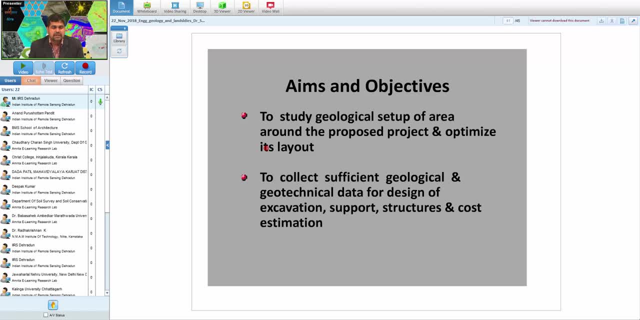 especially where people cannot go in regulations type of survey, satellite image is the best friend to tell you where exactly the alternate sites can exist. now, to collect sufficient, because you're not searching without field verification is nothing. so you have to collect sufficient geological, geotechnical data for design, designing of excavation, support structure and cost. 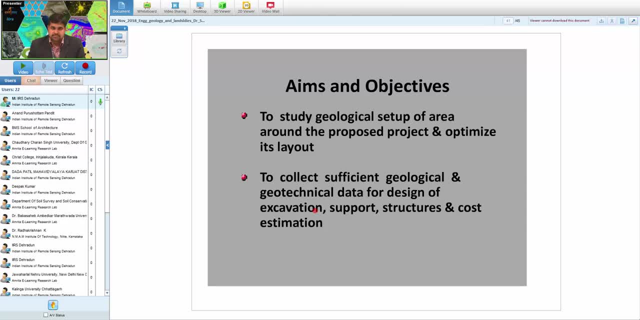 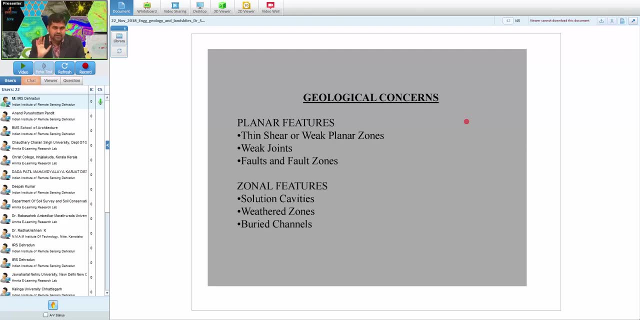 estimation. this part two, but this has to be done after your size primary facility has been selected. what are the geological concerns that we can add it to, that we can address using satellite data? so thin are series once we planes will joins, faults, fault Jones, using linear mint, using high resolution. 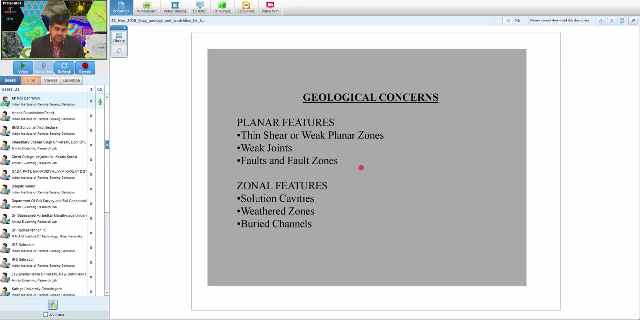 satellite data. a false curve can easily be diligent, get delineated in a cathode set one image, but it's a two images, so that will tell where exactly the weak Jones exists, without going to the field. as a Reiki kind of survey it can sub the. 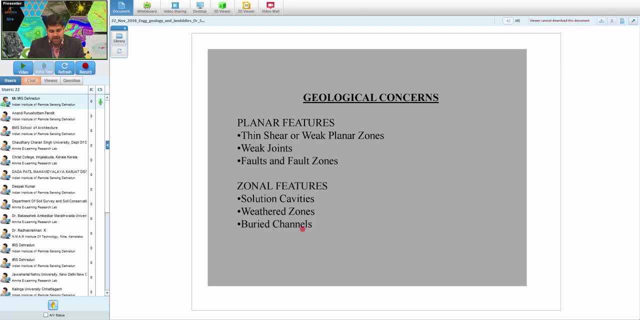 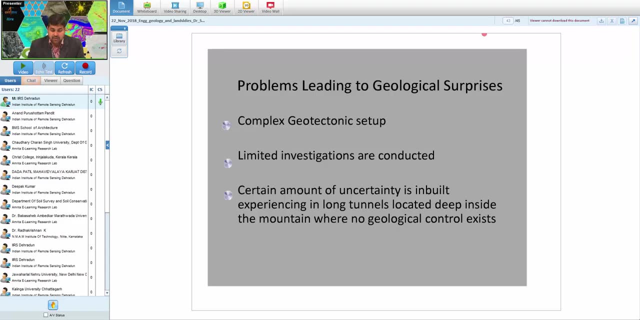 purpose, then obviously this required body channel, Psalm, somebody channel and satellite-based satellite scan analysis is going to help sports, an whether zones, solutions, cavities. this requires field verification also, but these are the studies that, these are the concerns that you have to consider before considering construction. 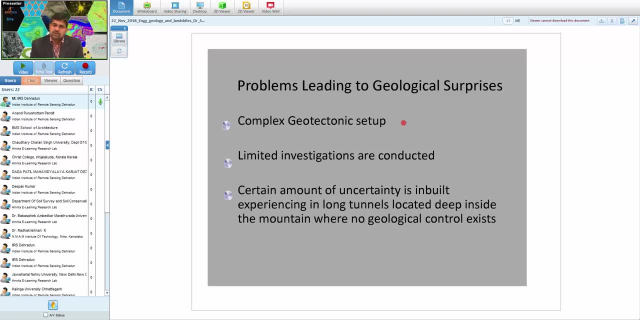 of a dam. What is the geological surprise? There is a term called geological surprise. we often come to know about this. What are they? Because, sometimes, including all these studies, your fieldwork, your civil engineering study, engineering geological study, remote sensing study, employing all these even if, when you 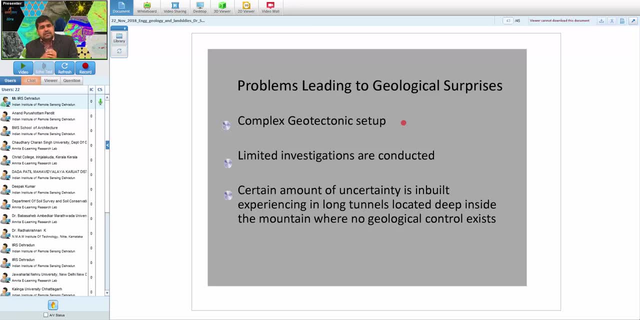 want to construct a dam or construct, a suppose, headrest tunnel, a tunnel. basically, there will be, geological uncertainties will be there. There can be a shear zone which you didn't expect, it didn't expect, but it is there. It cannot be, could not be projected from existing data. 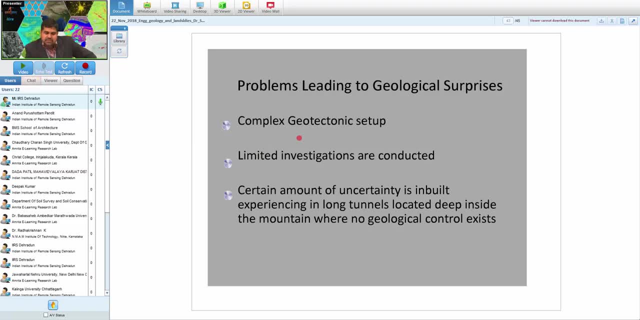 So that leads to the geological surprises. So this, basically, it is a result of complex geotechnical setup. because nature is nature, We have to understand that. sufficient clues We can get from satellite images and other ancillary features, but that cannot mimic. 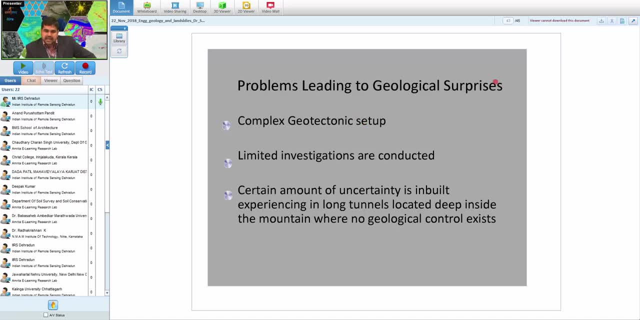 the nature in total. So there will always be complexities that will lead to geological surprises, Limited investigations- So this is another part- So if you do not have sufficient high resolution data, if you do not do ground validation, so limited investigation can tell, can lead to geological surprises. 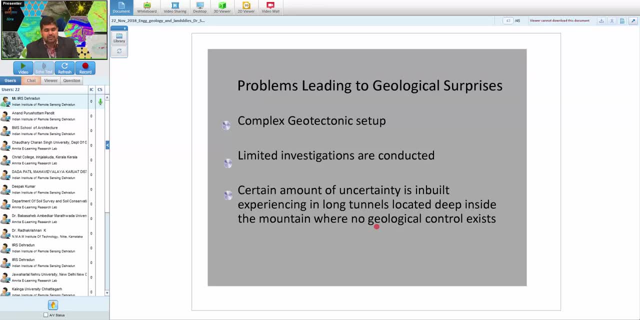 Certain amount of uncertainty in experiencing in long tunnels located deep inside the mountain where no geological surprises. So it is very difficult to know how geological control exist with the pressure. The in-situ pressure is so much So actually you do not have any geological control. 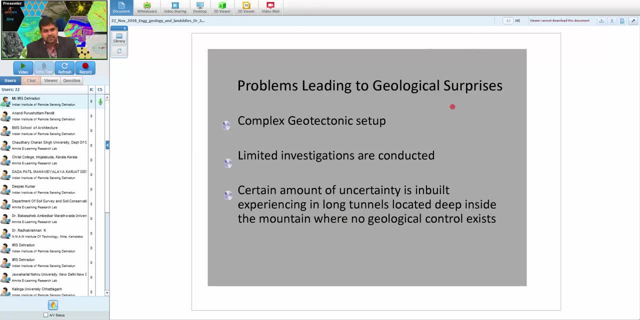 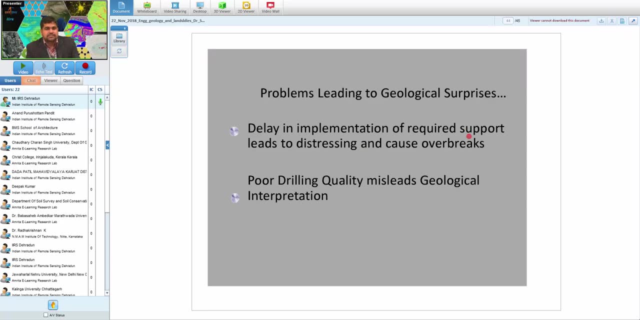 So that again leads to geological surprises. This is where we cannot help, Again delaying implementation of the required support. There is a suppose in a cavity you have made, a tunnel you have made, and you keep it like this without providing any kind of support. 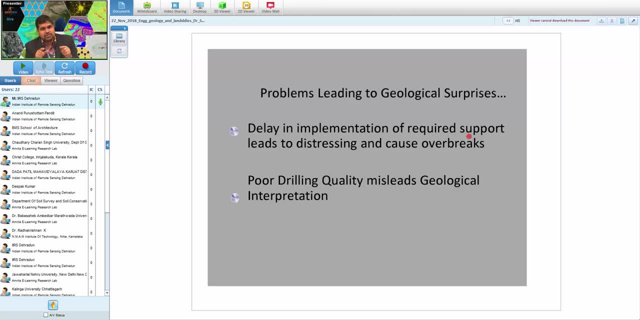 So there is a time, delay time, There is a time up to which, without any support, the tunnel will sustain itself by itself, so after that it will collapse. so for some rock it is immediate, so the time is very less. for some rocks it can be even years, even decades, so they are very competent. 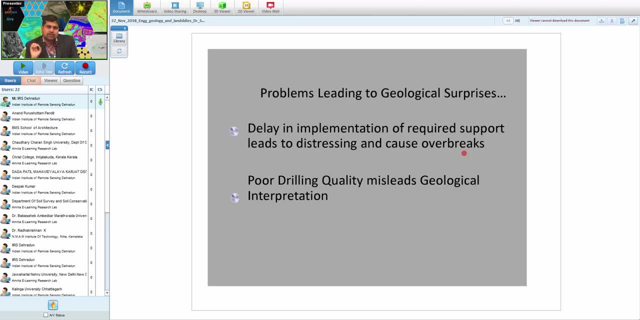 rocks. so that basically tells, if I can get to know about the, what type of rock it is, then immediately or in some time when this required, support has to be provided. without that there are chances that geological surprises will happen and poor drilling quality in. it is about ground validation, poor drilling quality.